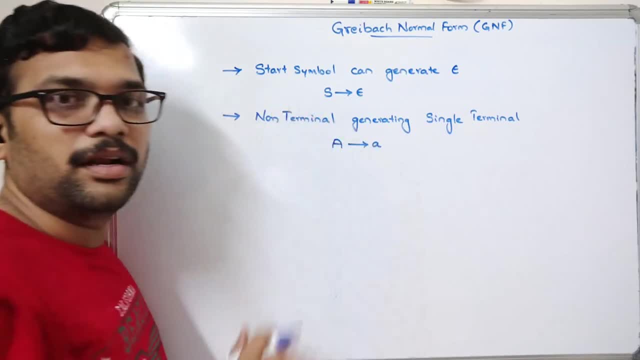 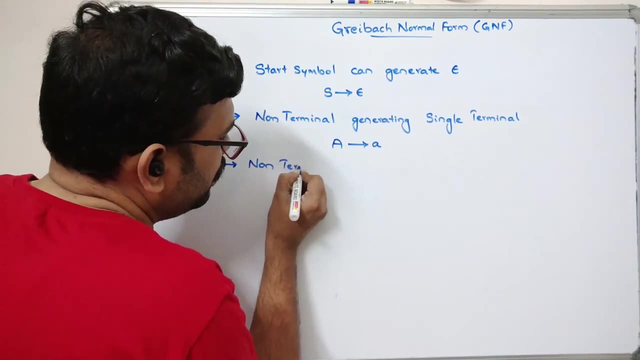 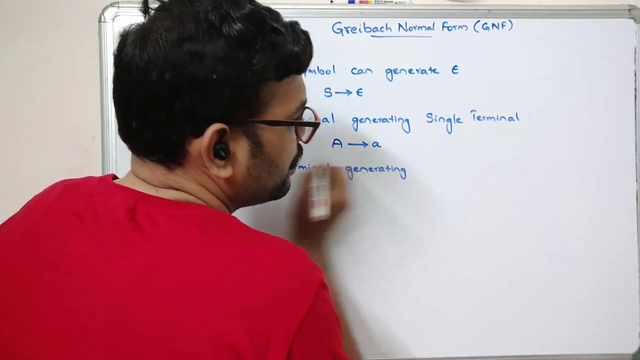 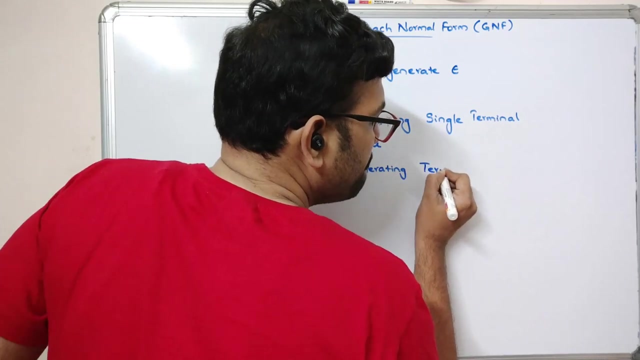 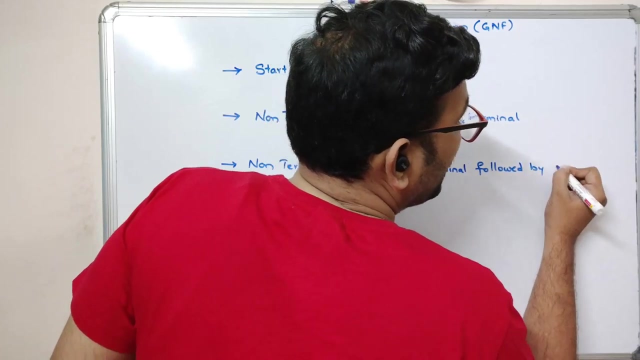 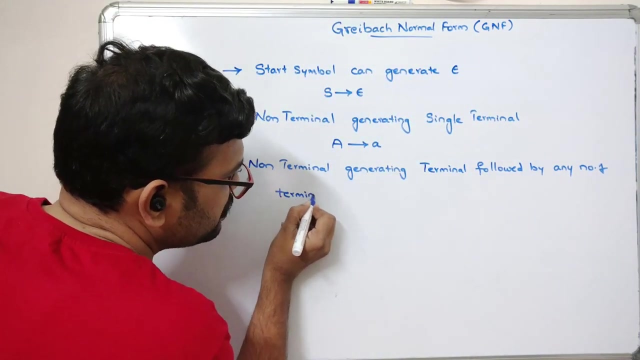 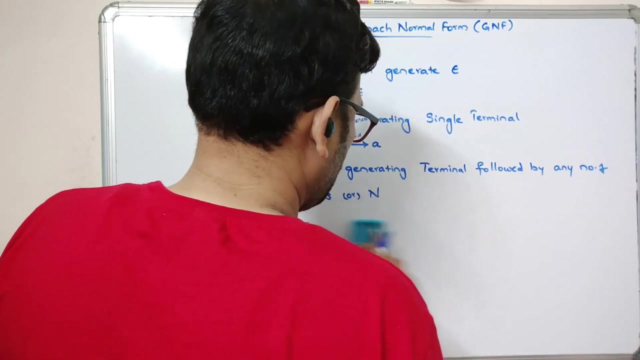 form, because the non-terminal generating the terminal And the third one non-terminal generating terminal, followed by any number of terminals or non-terminals. For example, let us take A- tends to B, So this is a non-terminal generating single terminal. 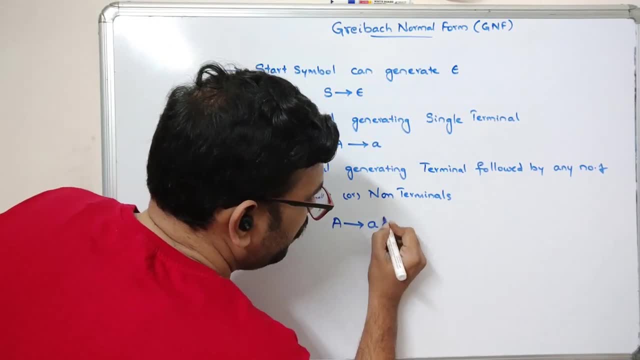 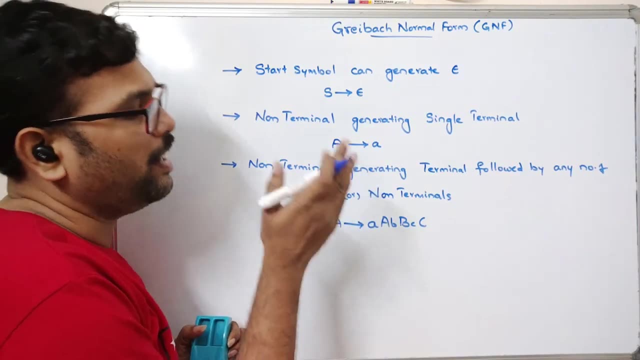 For example, let us take A tends to B, So this is a non-terminal generating single terminal. And the third one non-terminal generating single terminal, And this A tends to A, A, B, B, C, C, So this is also a valid production and this production is also in the form of grey batch, normal form. 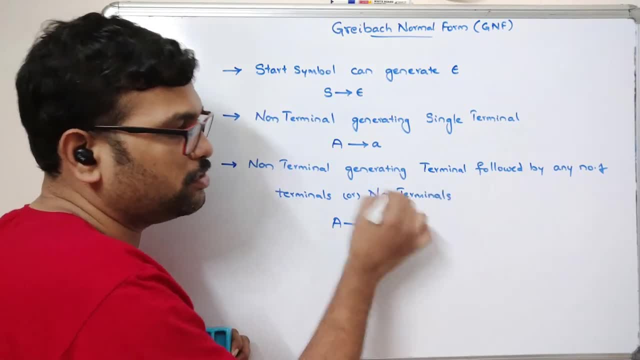 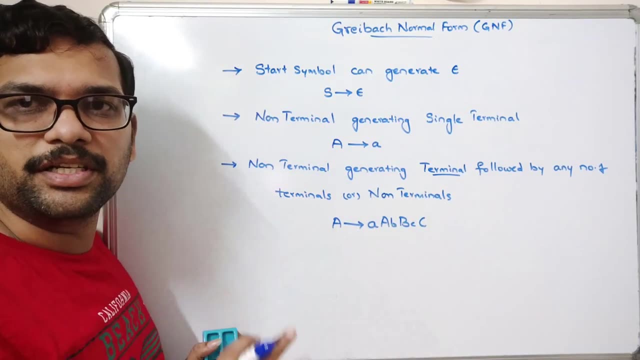 Because on the right-hand side of the production it starts, it should start with a terminal, followed by any combinations of terminals and non-terminals, Any combinations. it can be any combination, Any number of terminals and any number of non-terminals can be available here. 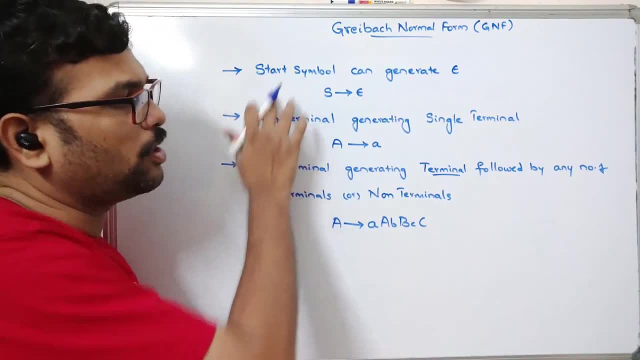 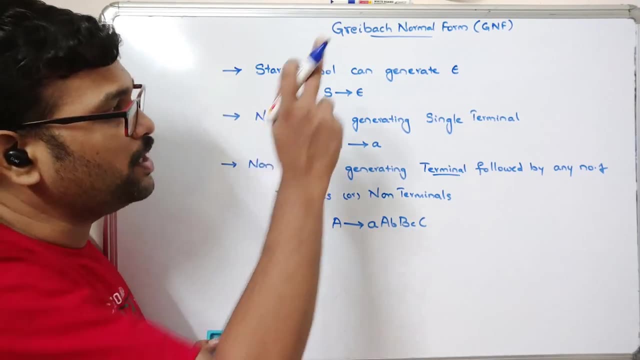 So if the productions are following these particular rules, then we can say that the productions are in the Gribach normal form, right? So hope you understood this one. First one, this is a start symbol with x1, which is similar to our Chomsky. And the second one is also. 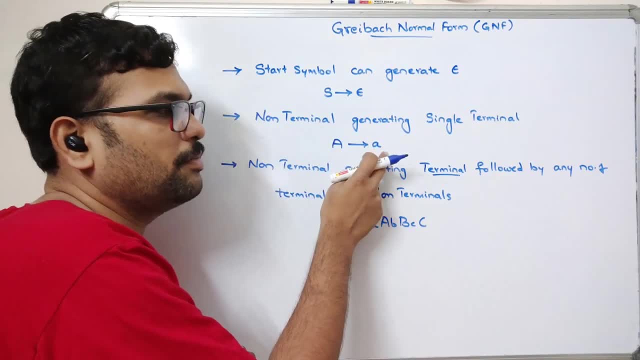 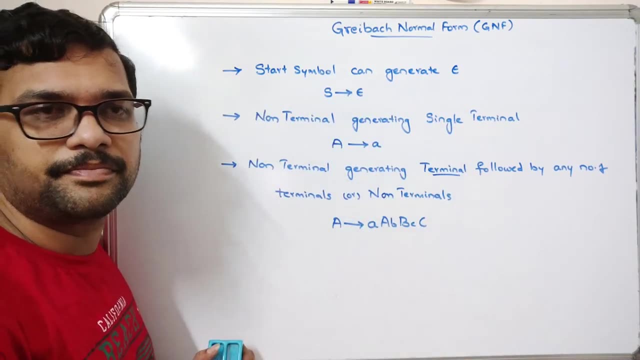 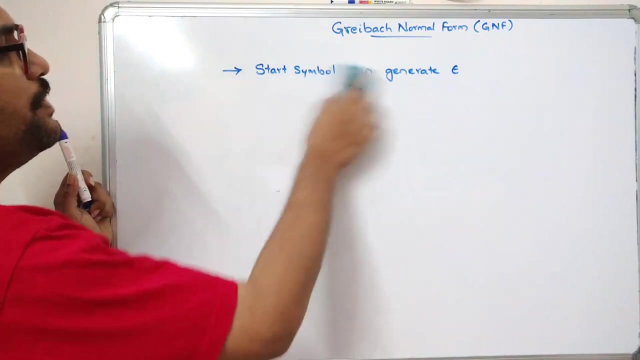 similar to our Chomsky. that means the non-terminal generating a terminal And the third one, a non-terminal generating a terminal, followed by n number of terminals and non-terminals. right Now we will see the steps to be followed in the conversion of context tree driver to: 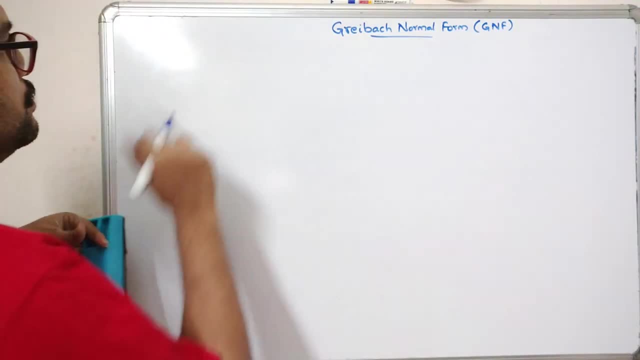 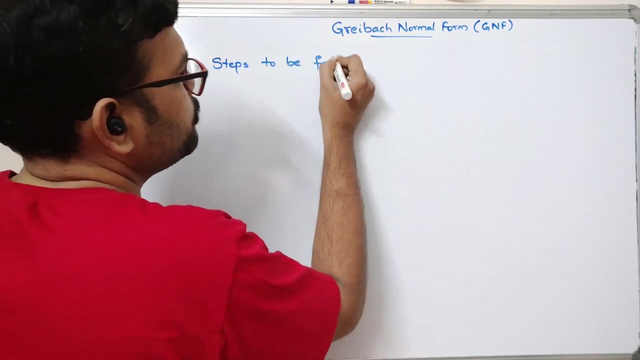 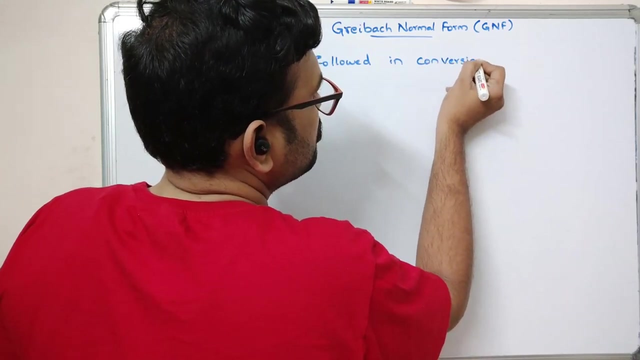 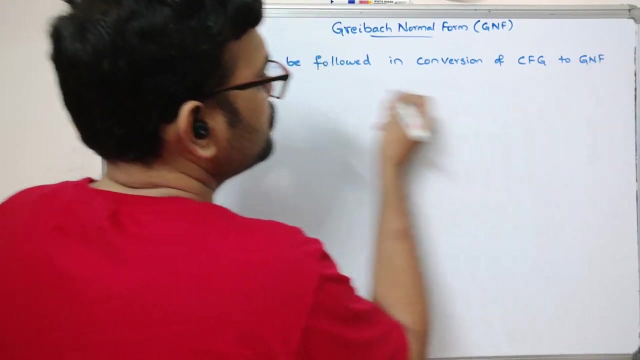 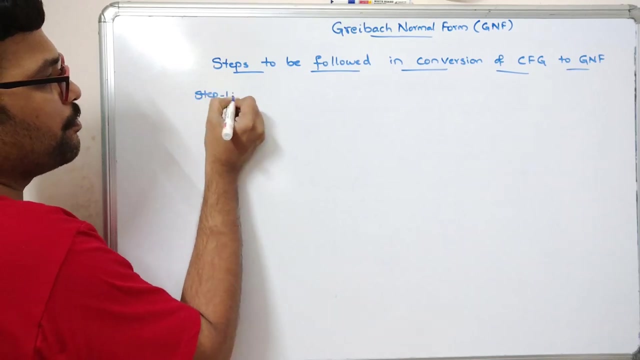 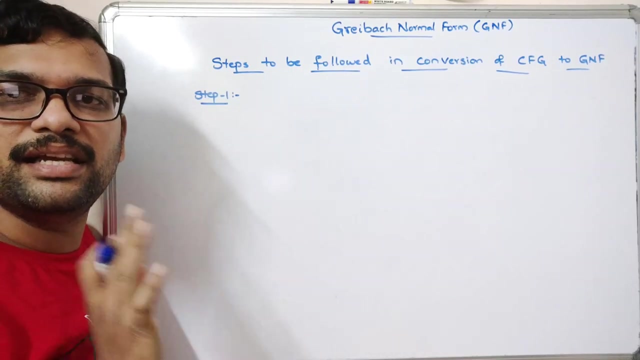 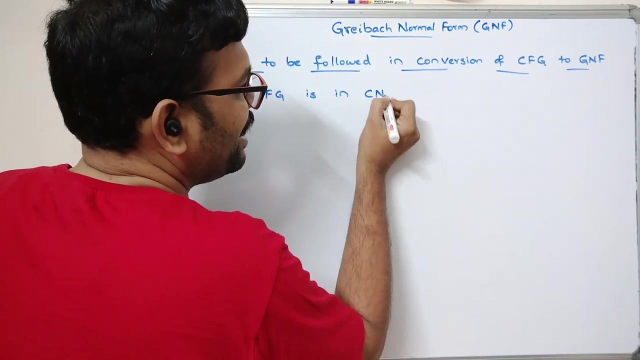 Gribach normal form. Steps to be followed in the conversion of C of G to G of G. So G of G is Gribach normal form. So step one, step one. the step one is make sure that the C of G is in a C of F. okay, C of G, given C of G is in C of F. So this video we already. 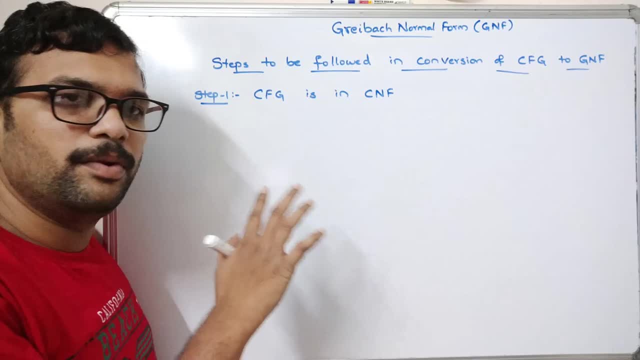 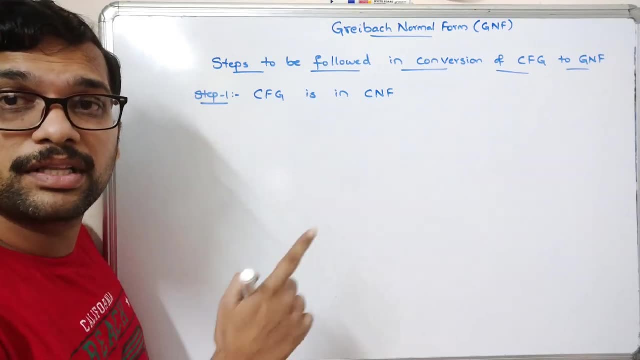 we have covered in the previous session this topic, So I will post the link in the description so that you can follow that. So first step: the C of G must be in C of F. If not, you have to convert the C of G into C of F first. 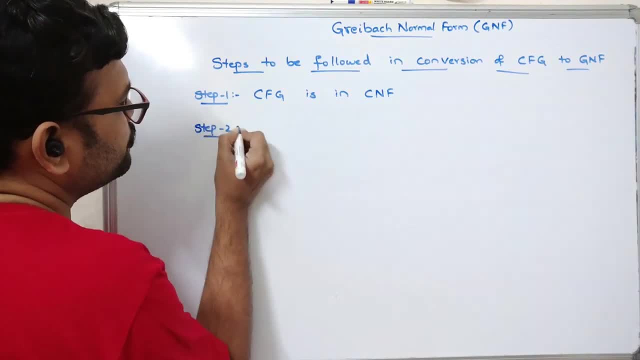 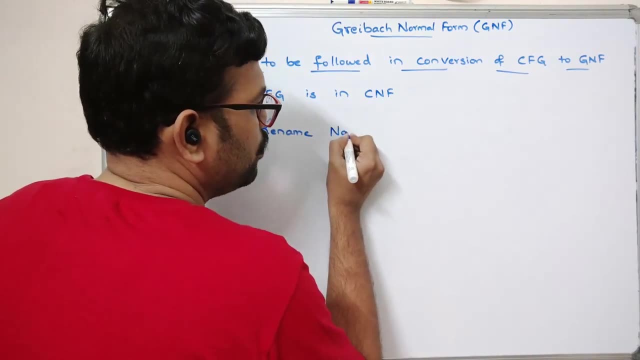 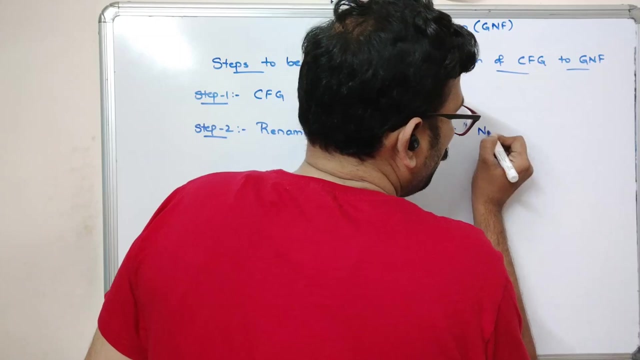 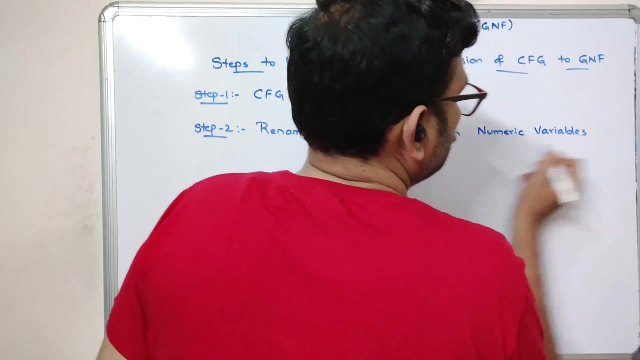 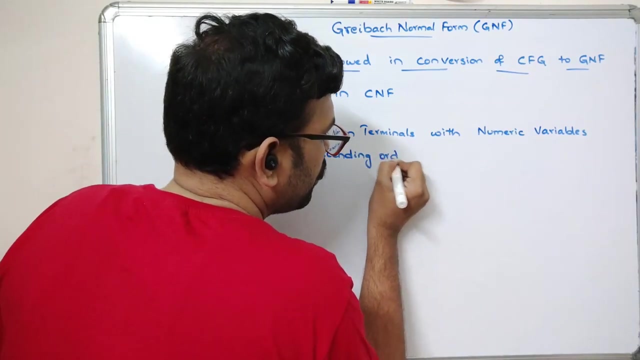 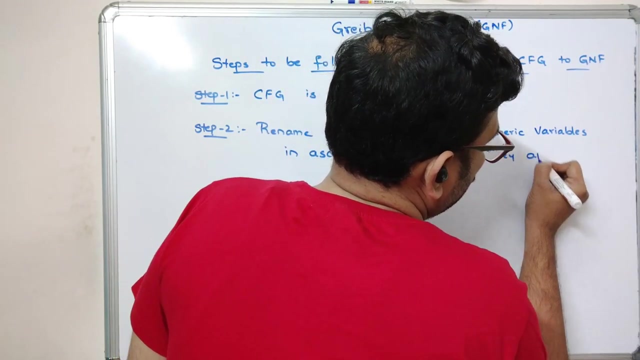 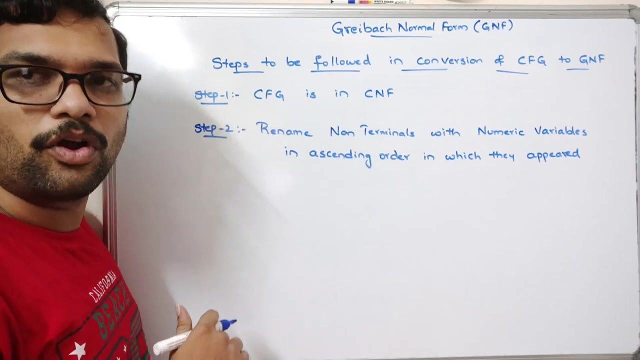 Then step two: rename. rename non-terminals with non-terminals with numeric numeric variables in ascending order in which they appear. okay, So first one is we need to rename the non-terminals with terminal, non-terminal numeric variables, right? For example, if our 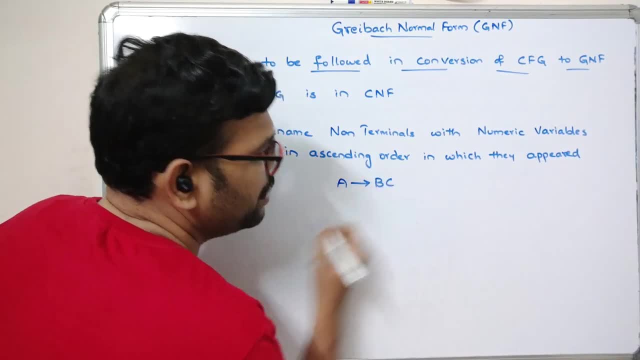 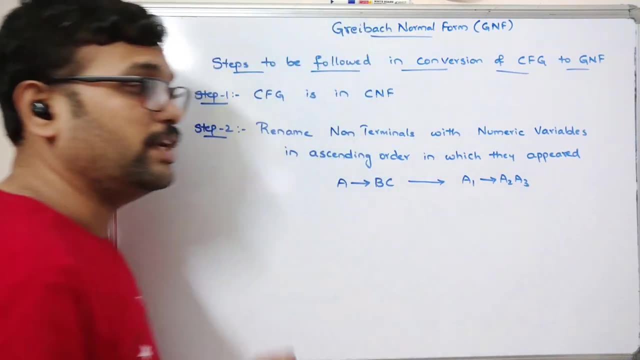 production is having some A tends to B, C, So rename this one with A1, tends to A2, A3. So that means we need to rename the non-terminals with any name with a numerics. okay, Let it. 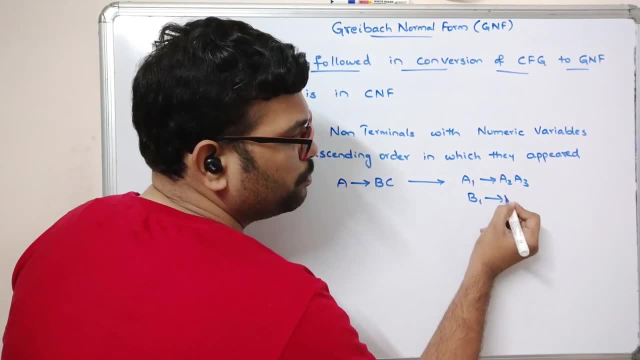 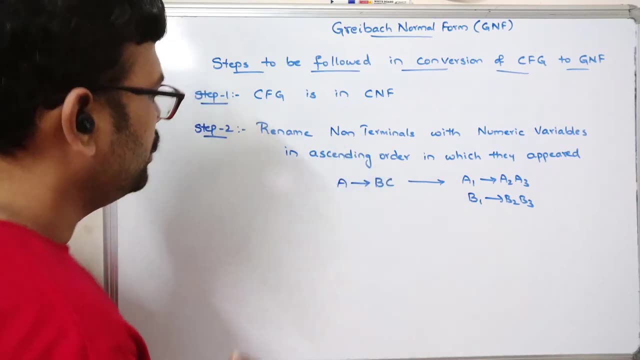 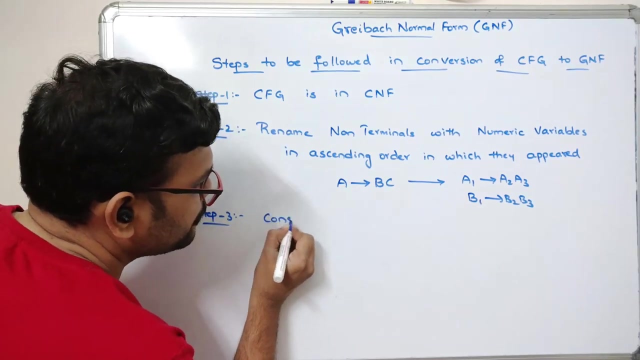 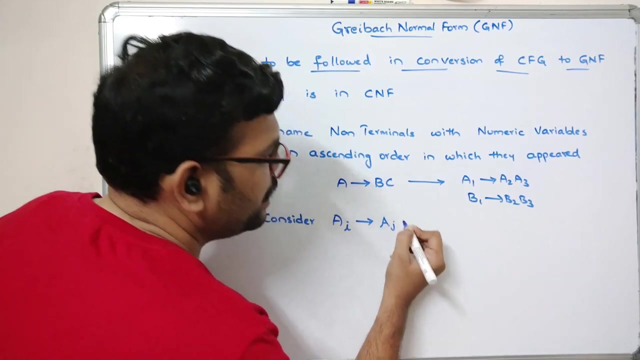 be A1 tends to A2, A3, or B1 tends to B2, B3. So any name, you can take any name, but just use the numbers numeric variable. Then step three. So consider, consider A, I tends to A, J and so on. right Now there can mean. 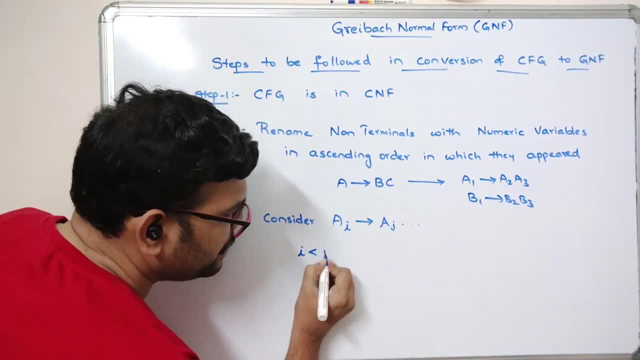 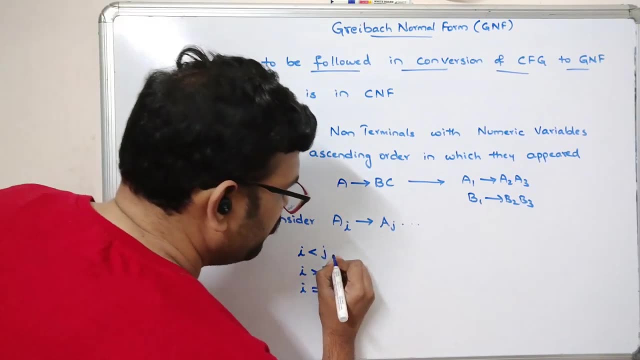 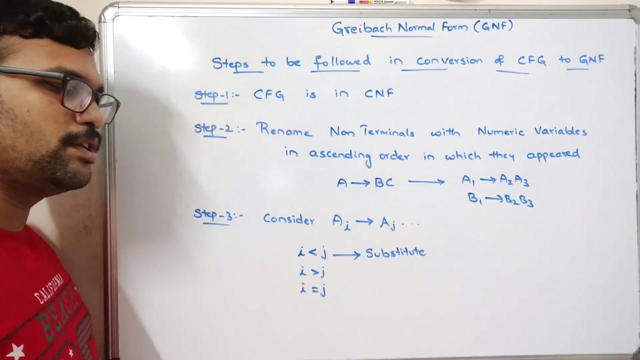 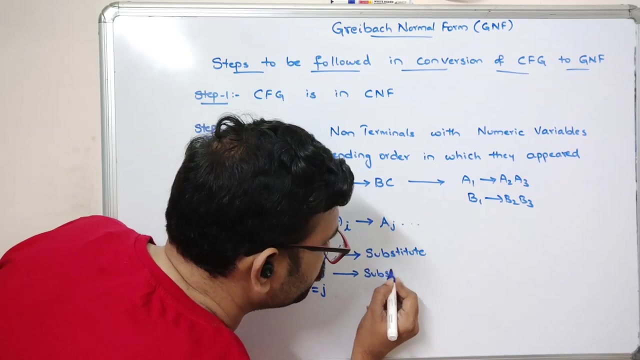 a comparison between I and J. So I ridiculous care- I is equal to J. okay, So if I is experience A, just use the substitution method. Use the substitution method, Substitute one production in another production, And if i greater than j- here also, you can simply use the substitution. 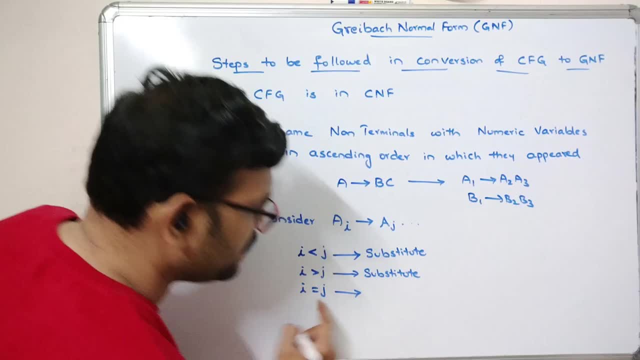 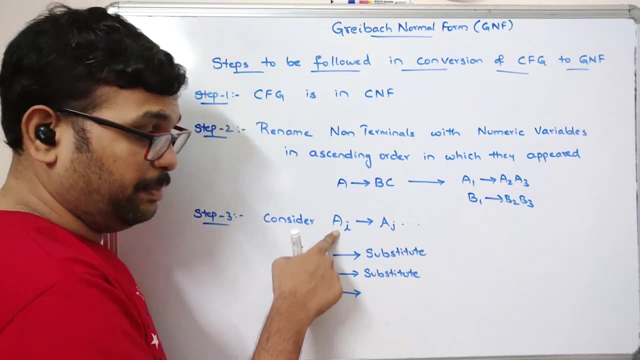 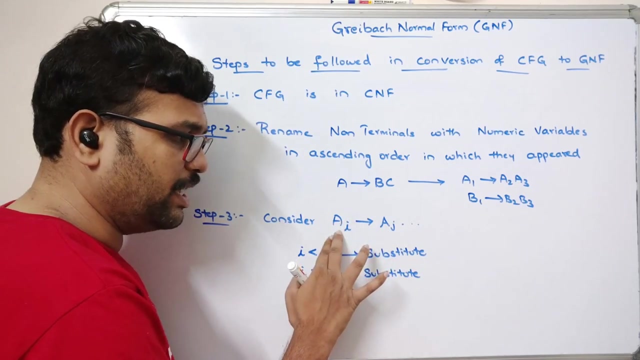 method And if i is equal to j, you can see that i tends to aj. if i and j are equal, Okay, That means both the non-termals are equal And you can see on the left hand side, whatever the non-termal is there on the right hand side, you are having the same non-termal on the left. 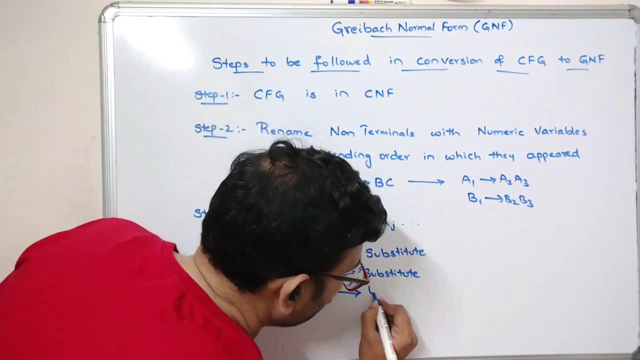 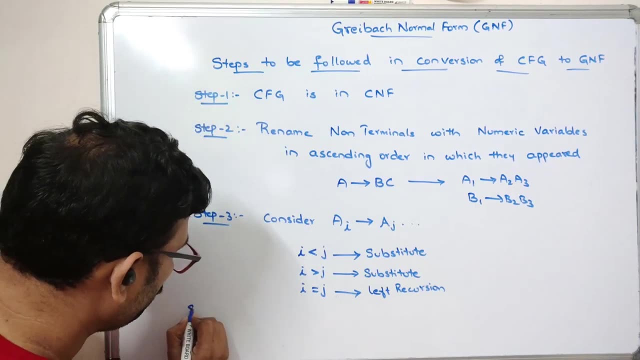 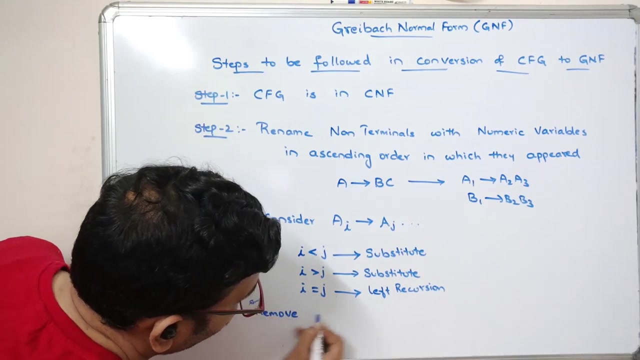 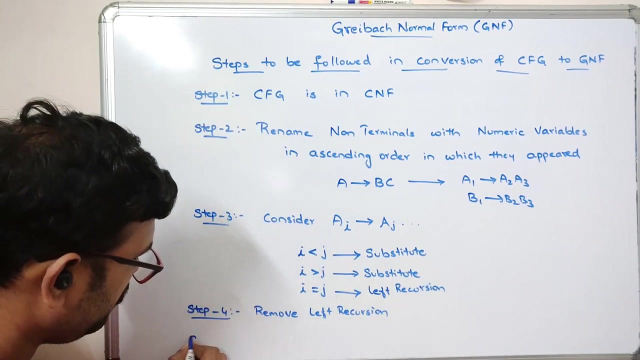 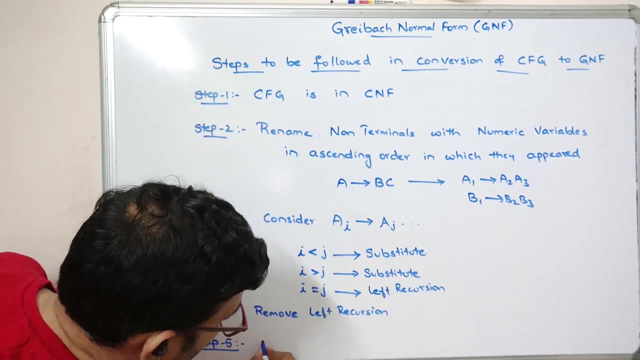 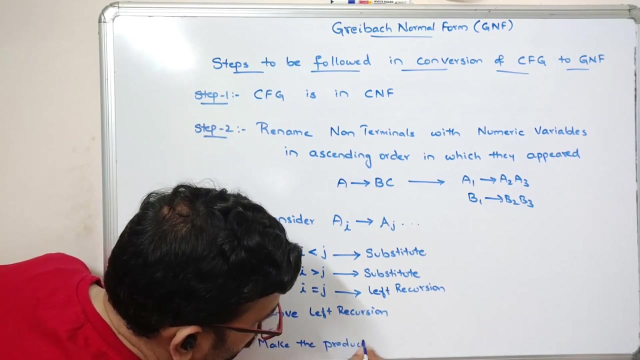 most, So that is called a left recursion. Okay, So this is the left recursion, This is the left recursion. So the step four: Remove left recursion And remove left recursion. The last step, Step five: Make the productions follows or following. 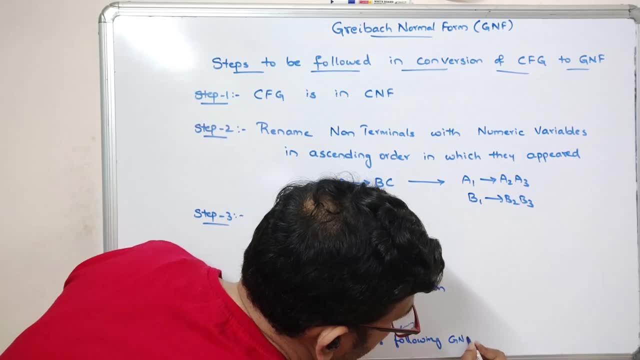 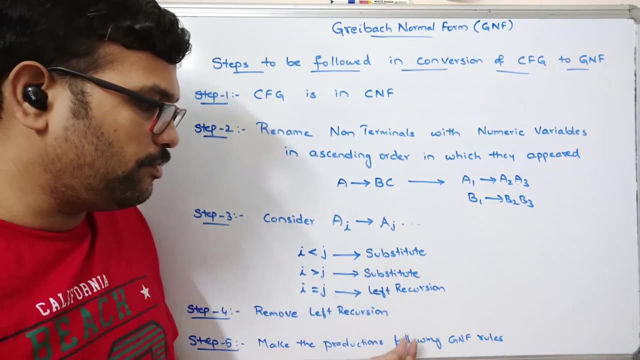 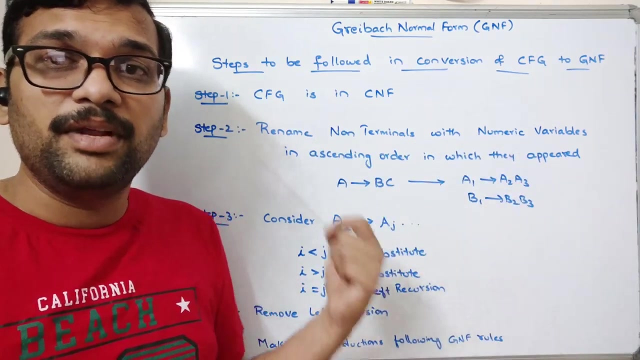 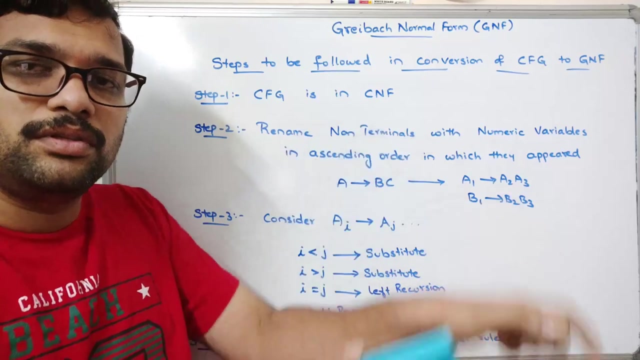 GNF roots. So use the substitution methods and make the productions that following the GNF roots. That means the non-terminal generating the terminal and non-terminal generating a terminal followed by n number of terminals and non-terminals. So we have to make the productions to such 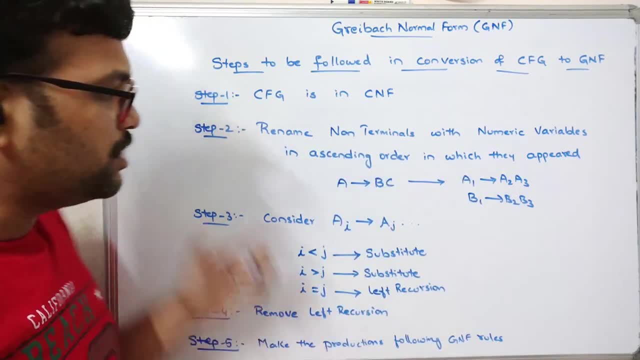 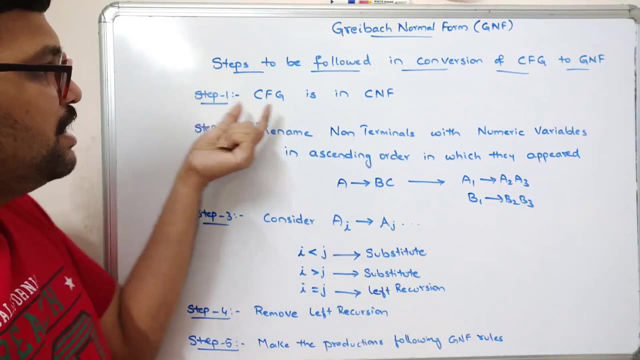 productions which obeys these rules Right. So these are the steps we need to follow while converting the CFG to GNF Right. The first one: the CFG must be in CNF. If not, you have to convert the CFG into CNF first And second. 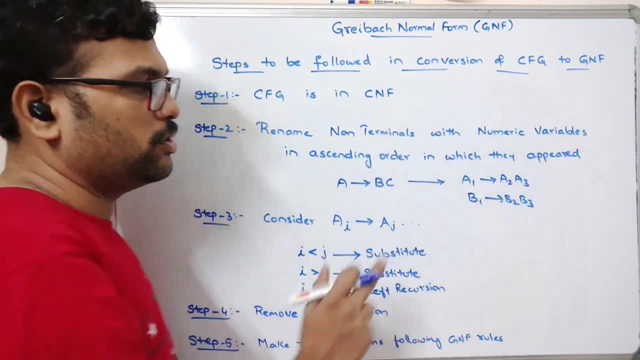 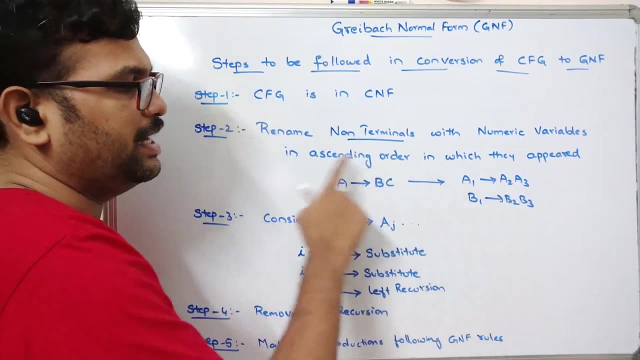 rename all the non-terminals which are available with a numeric variables, Only the non terminals. Right: only the non-terminals. So with the numeric variables. that means variables will be numeric in ascending order which they appear. So your, your having ABC, So a will be replaced with A1.. 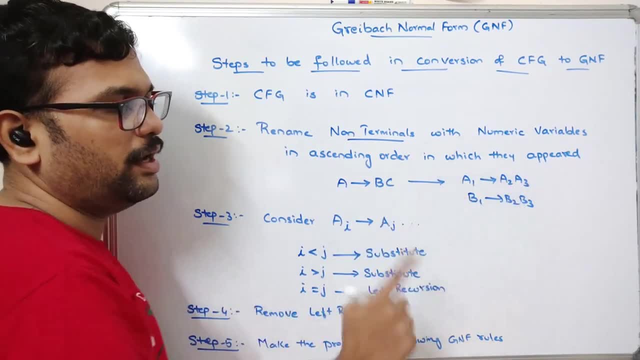 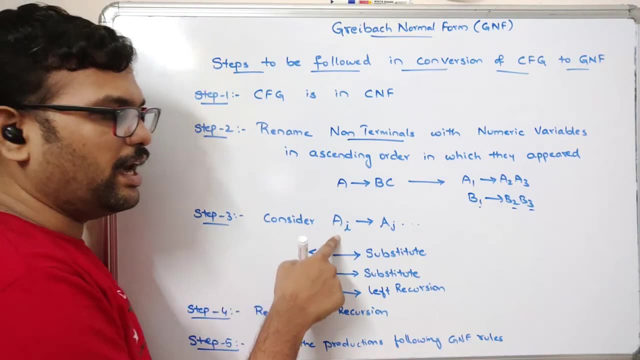 BC too, mm. Or you can also replace it with any other names, But numeric is important. And in the next step, consider: AI is generating Aja, followed by the. I still never thought about name Any any other reasons or these words may take longer. 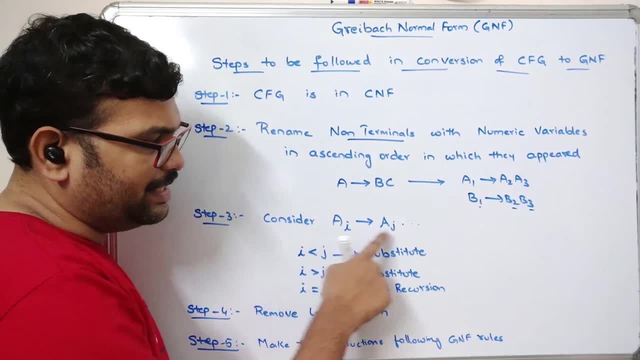 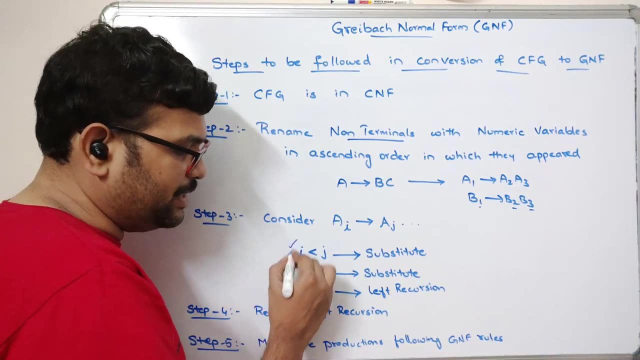 string. So then we have to compare the i and j values: i less than j, i greater than j and i is equal to j. So three combinations from beginning. So if it is i less than j and i greater than j, you can use a substitute method, And if i is equal to j, that is nothing but a. 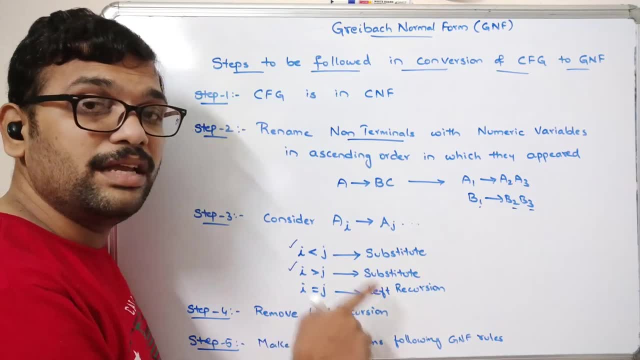 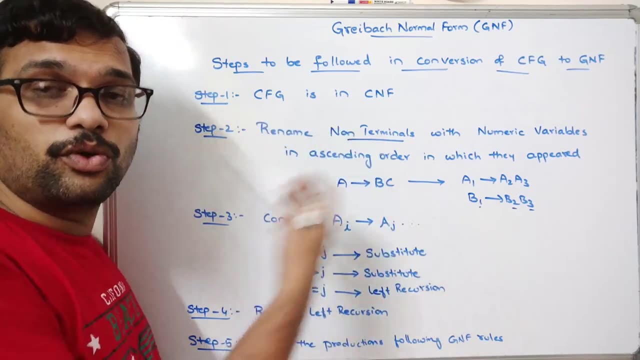 left recursion. So step 4, we have to remove the left recursions, if any left recursions appear here. And step 5, we have to convert the productions to the productions which obey the GNF rules right. So we will see the example so that you will be understanding all these steps. 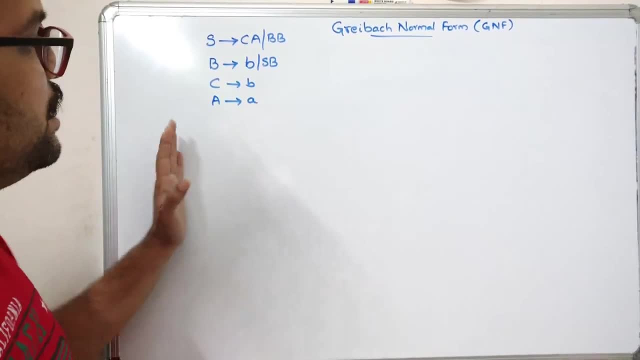 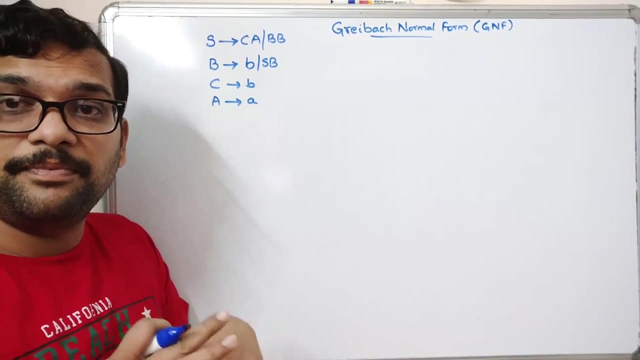 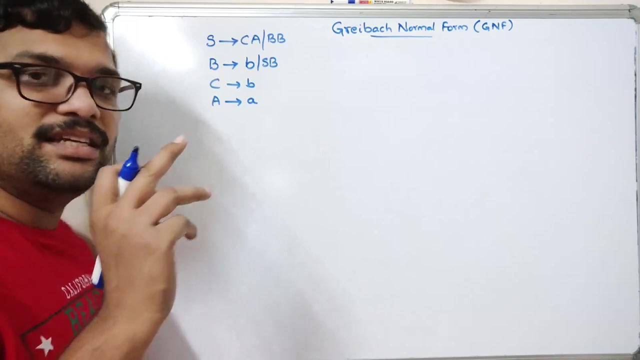 right. So let us take this example. So this is the CFG given and we need to convert this context-free grammar to GNF. So what is the first step? We need to check whether the CFG is in CNF or not. If not, we need to convert it right. So first let us check. So in the CNF. 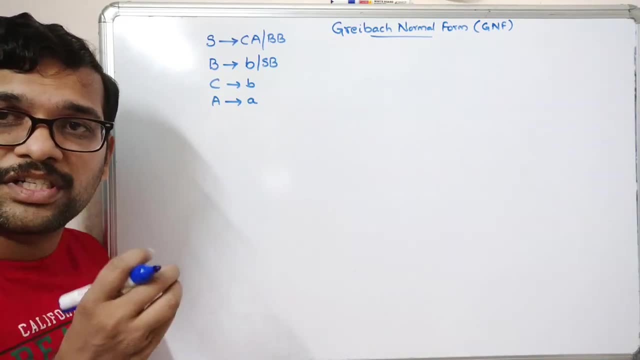 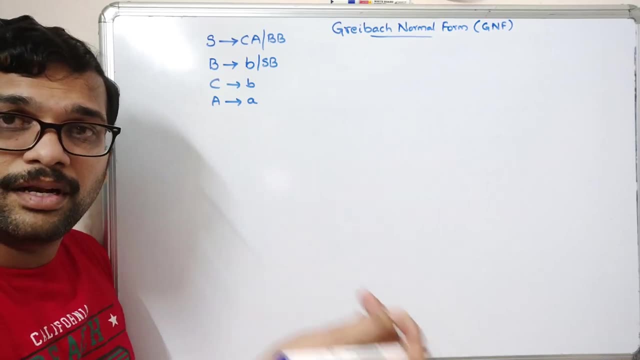 we know that Chomsky normal form, we know that the productions must be the start. start symbol can have the epsilon and the non-termghan will can generate a terminal and non-term orthogonality must generate two non terminals, exactly two nonてhnasaki need. 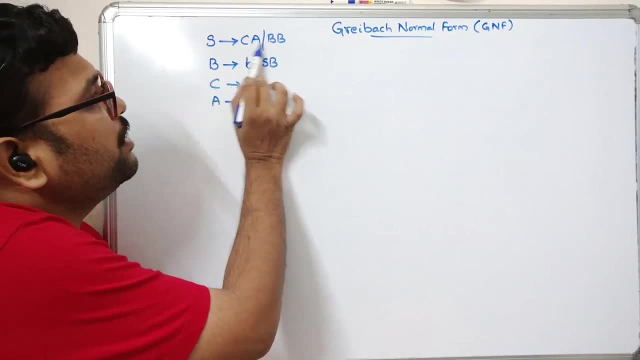 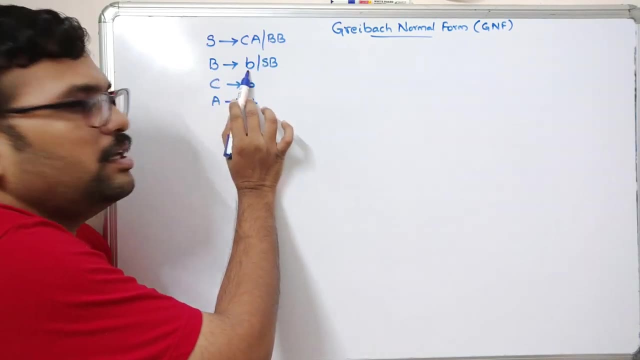 were two non terminals. So you can see here and non-termindre generating two, exactly two non-terminal. so this, this production, is in CNF and again here, the non-terminal generating terminal, it is in CNF, Non-terminal generating two. 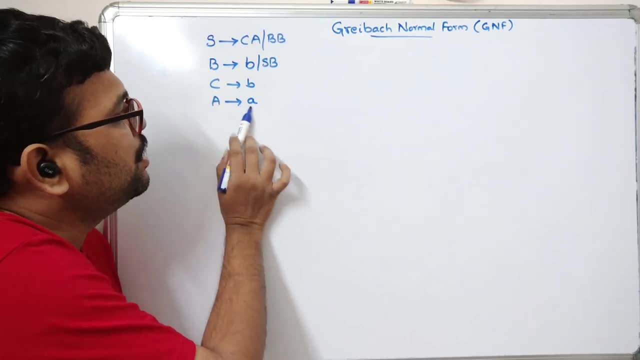 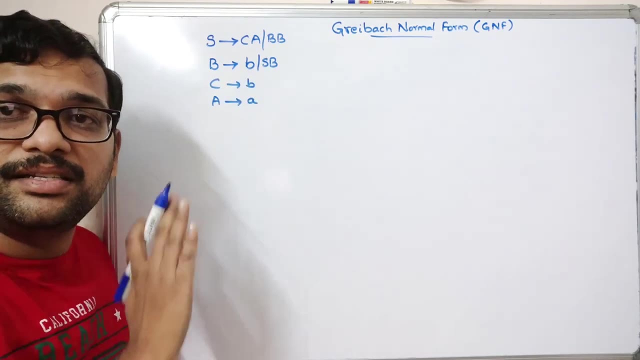 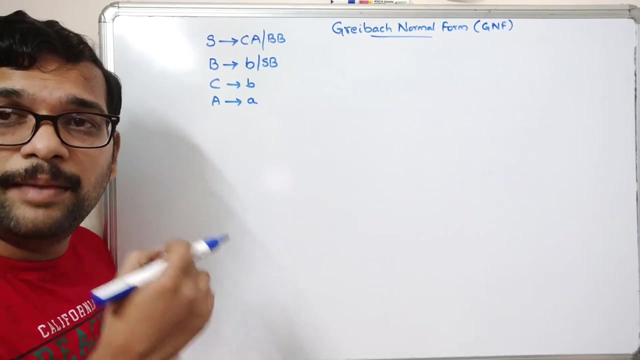 non-terminal. he is in CNF, Non-terminal generating a terminal. so these are in CNF. So we can see that the given context with grammar is in CLF. so we can avoid the step 1, there can be the step 2, so what is the step 2 here? so we need to rename the non-terminals with. 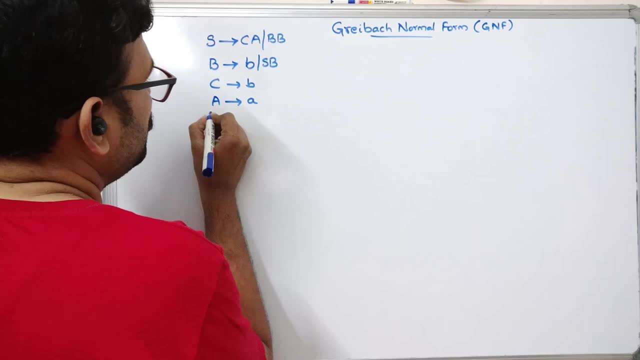 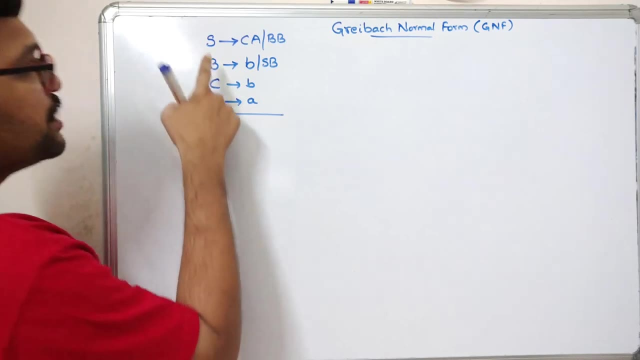 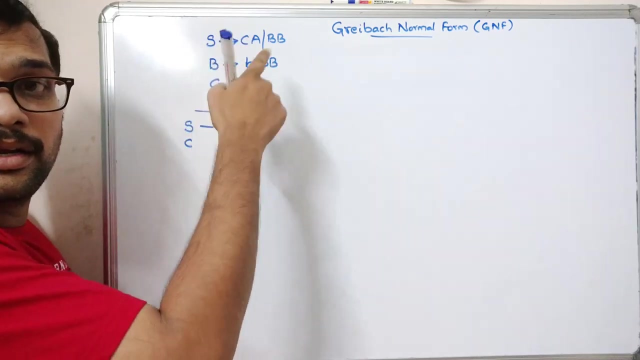 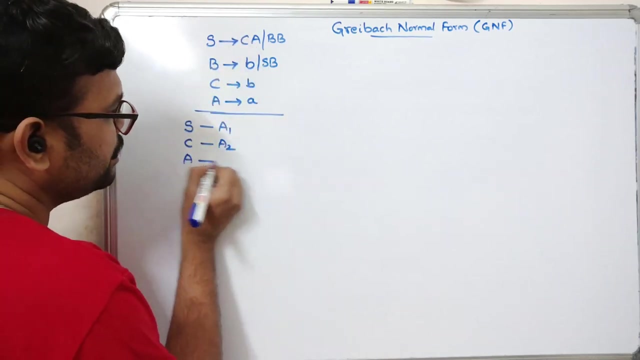 the numeric variables right. so let us take ascending order. the first non-terminal is yes. yes will be replaced with a1, next c. so just follow the order right in which they appear. so next one is c. c can be replaced with a2, a is replaced with a3, b can be replaced. 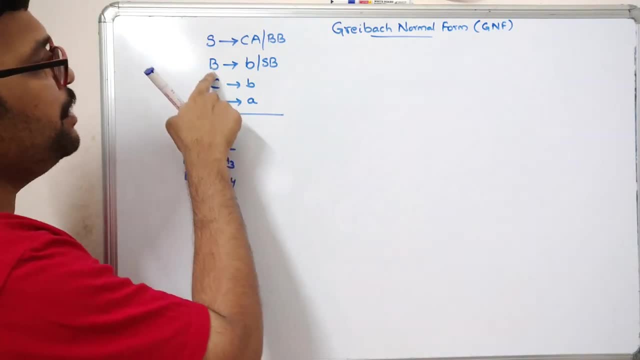 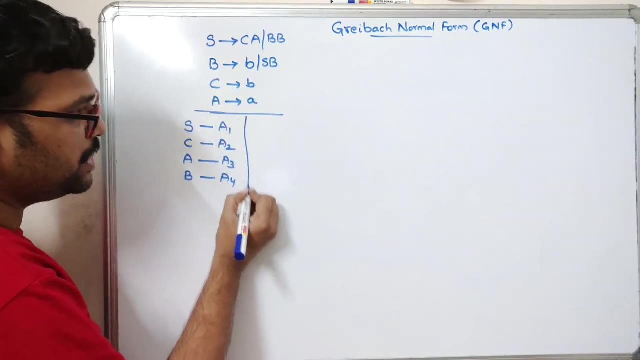 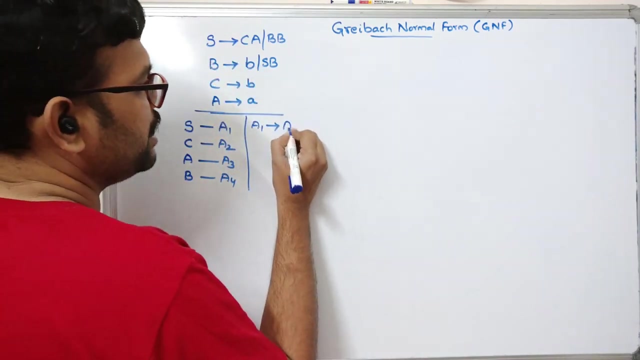 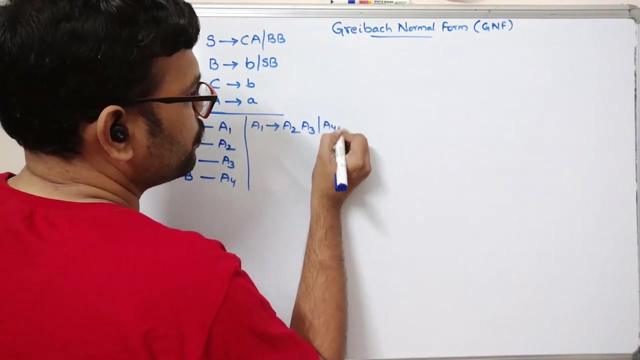 with a4, okay. and again b already renamed, and, yes, already renamed, b already renamed, now just apply this one. so a1 tends to what is the c, it is a2, what is a, it is a3. or bb. bb means a4, a4, similarly. 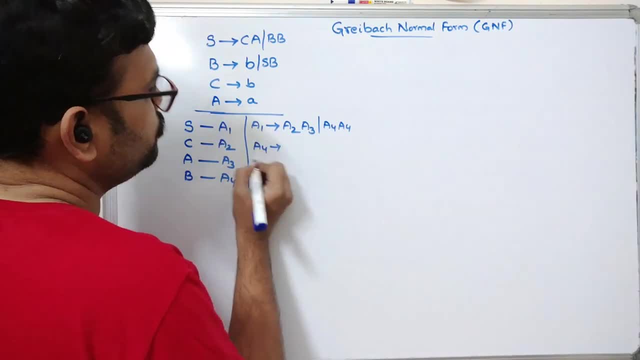 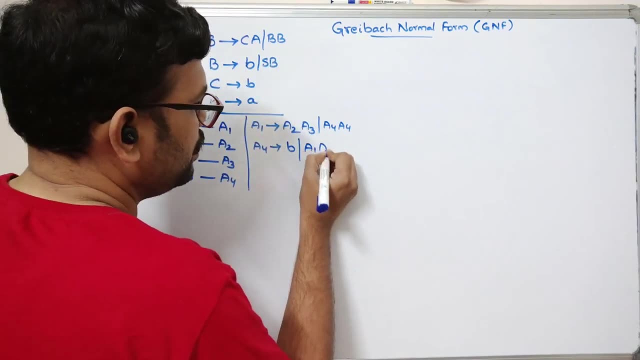 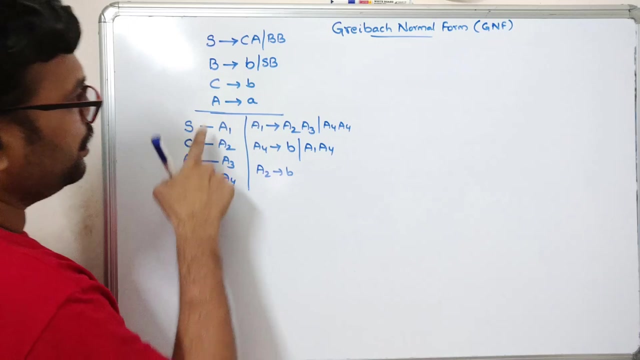 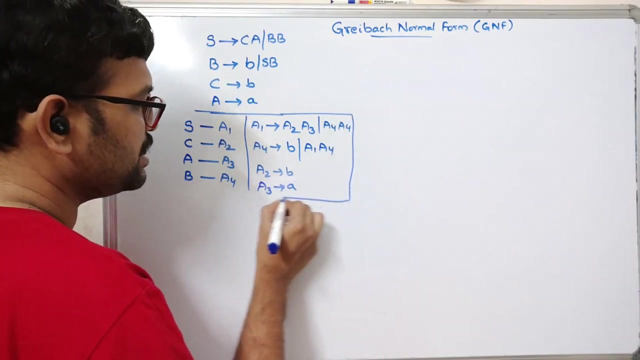 next b. b means a4 tends to b, or yes, it is a1 and b it is a4, and similarly, c means a2 tends to b, And here a means a3 tends to a. right now, you can observe, this is our cfg, this is our. 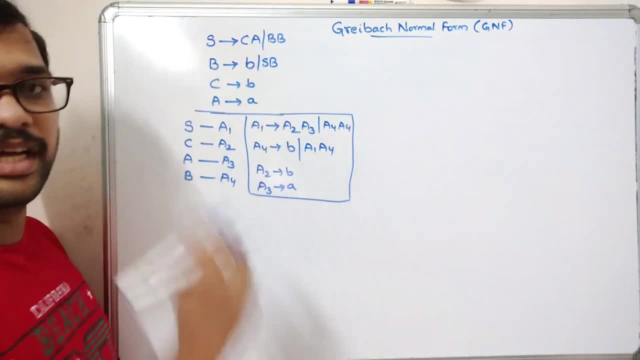 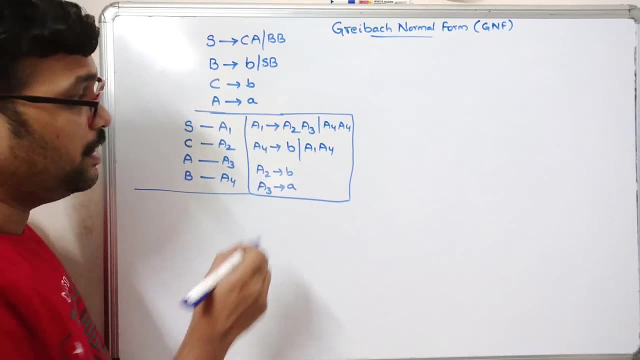 cfg and we need to convert this one into gen now. now, so what we have to do? so consider i and j, i and j, and here you can observe i is 1 and j is 2, in this production, you. 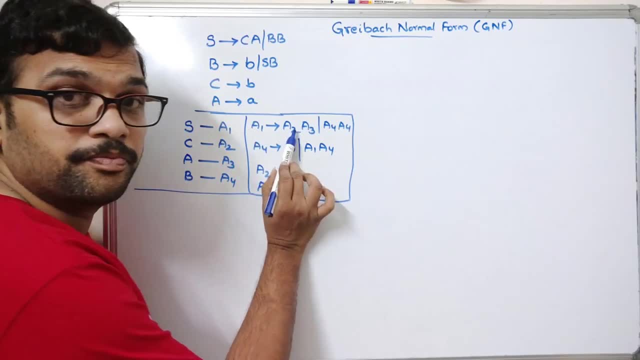 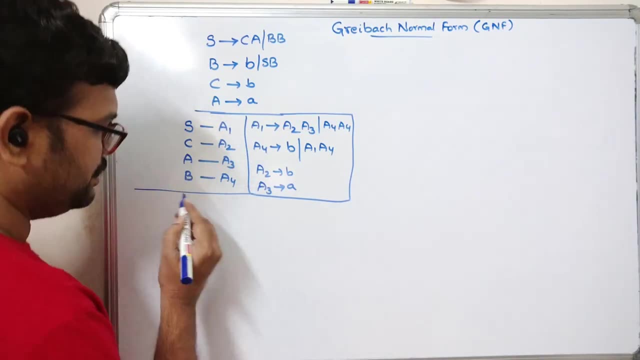 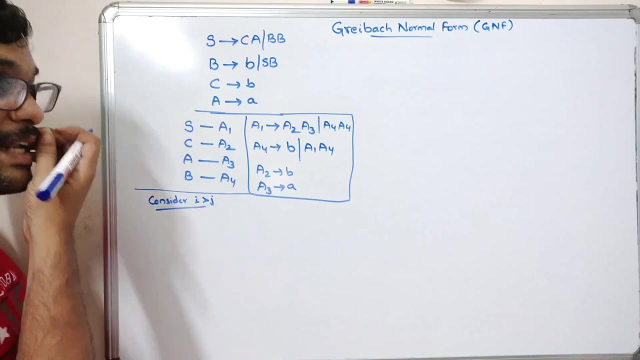 can see, i is 1 and j is 2.. But one include less than 2,. 1 is less than 2,, so you can simply substitute it, or so. first consider the i greater than j. i greater than j. first consider the i greater than j. so 1, i is 1 and i is 2, 1 less than. 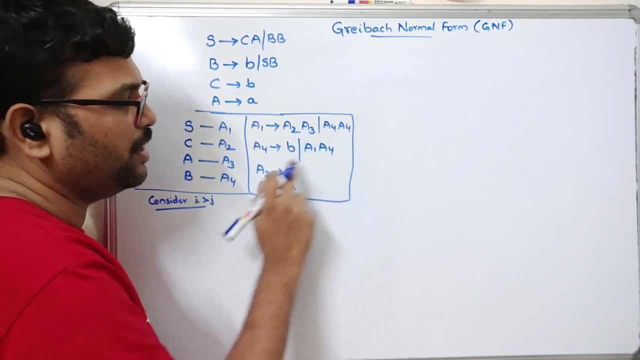 2, so just leave it 1 less than 4,. just leave it 4 less than 1, so that means i greater than j. So consider this production a4, a1, a4, a1. now what we have is a2, a2, i, a4, a3, so 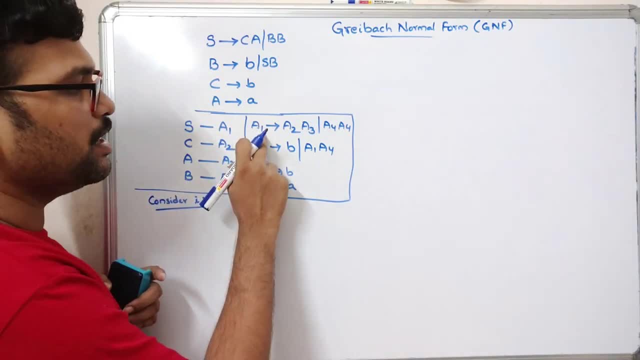 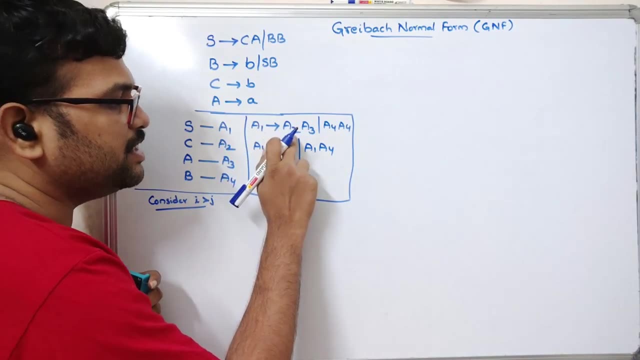 we can substitute it a1 less than j. Hope you understood this one. So let us consider this one as i and this one as j. Here i is 1 and j is 2.. So i less than j. So first we will consider i greater than j. So. 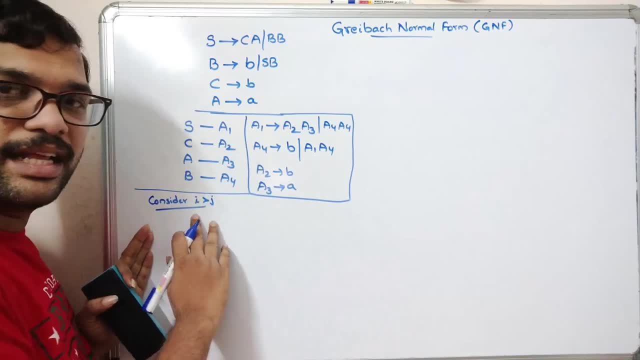 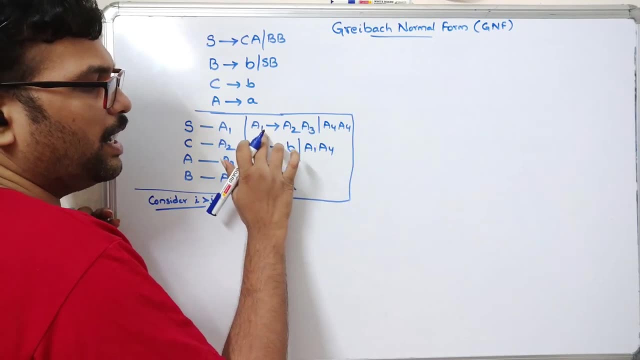 even though i is less than j, we can simply substitute: First we will consider i greater than j, then i less than j, and then i is equal to j. So you can observe here: i less than j, Leave it, And i less than j. So this is one more production. a1 tends to a4, a4.. So 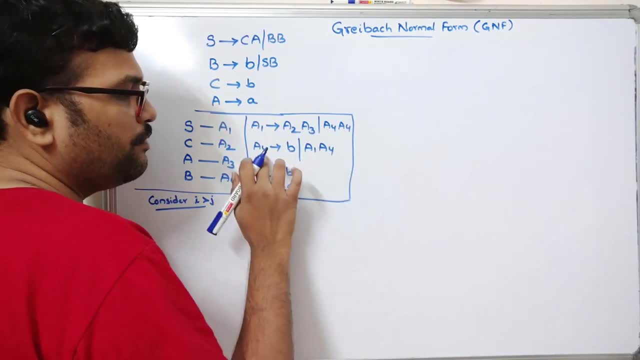 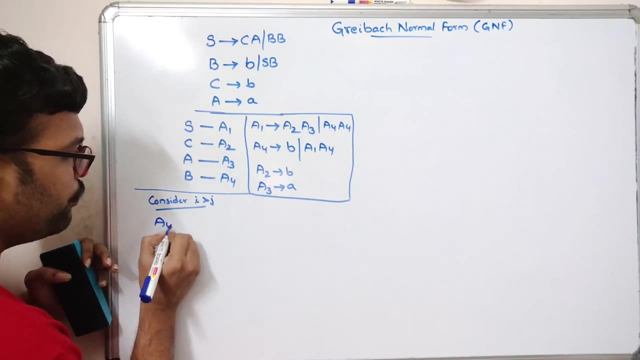 i is 1 and j is 4.. 1 less than 4.. Again, leave it. 4 tends to 1.. So 4 is greater than 1.. So i is greater than j, So consider this one. So let us take: a4 tends to b, or a1, a4.. 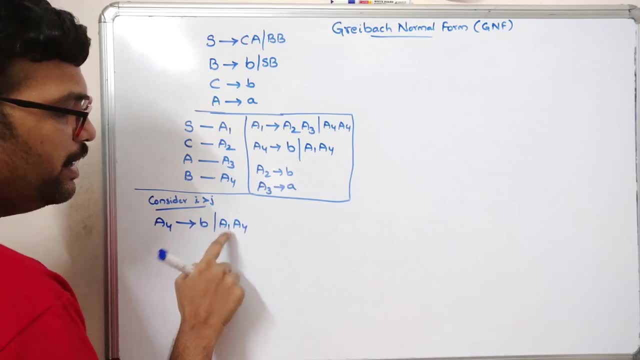 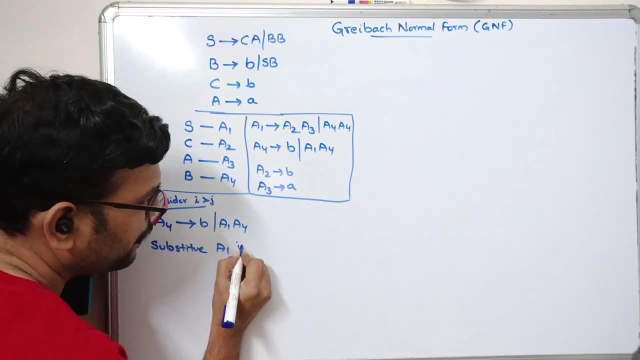 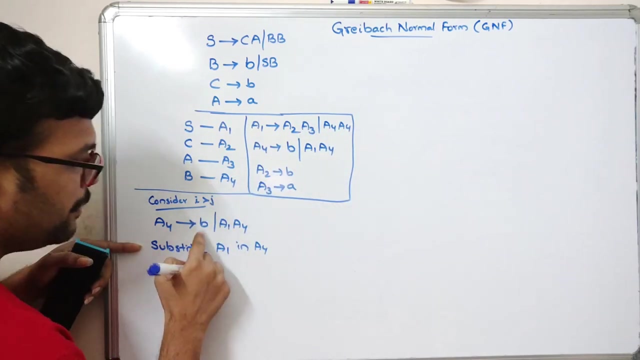 And you can substitute the a1.. So a1 here itself. So substitute a1 in a4.. So what is a1 here? a2.. a2, a3, a4, a4. Now a4 becomes b and in the place of a1, we need to substitute this one. 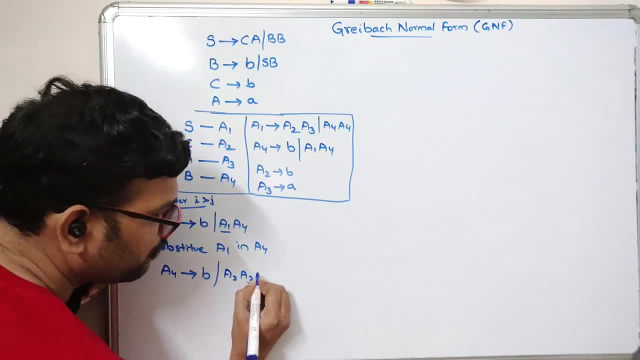 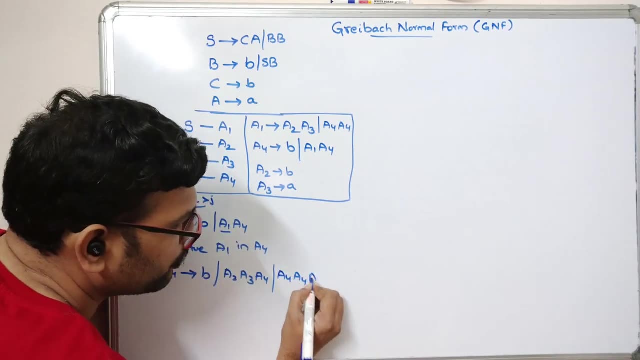 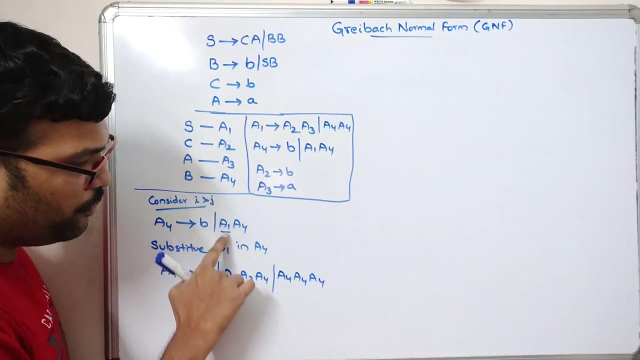 So a2, a3 and just write down this a4 and a4, a4 and just write down this a4.. So hope you understood. Instead of a1, we are writing a2, a3 and a4, a4.. So a2, a3 is a1. 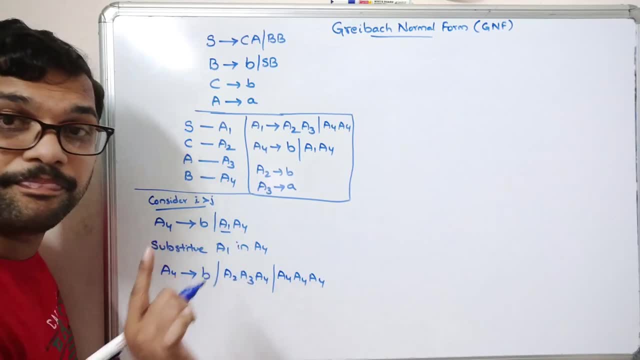 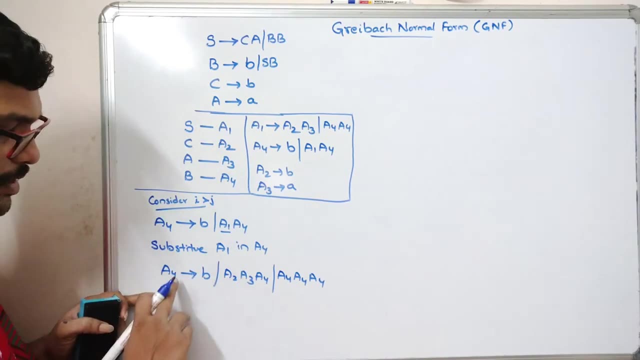 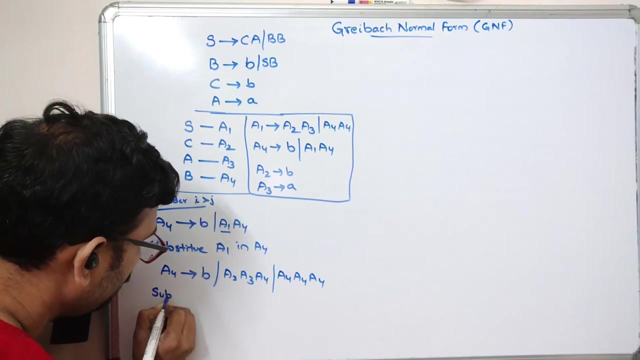 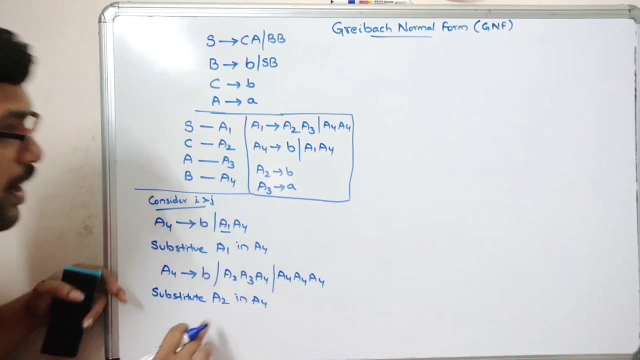 and a4, a4 is a1. So this a4 will be remained. Next consider again i and j. Consider i and j, So 4 and 2.. So greater than Okay, 4 is greater than 2.. So here again, substitute a2 in a4. So you can see a2 tends to b here. So 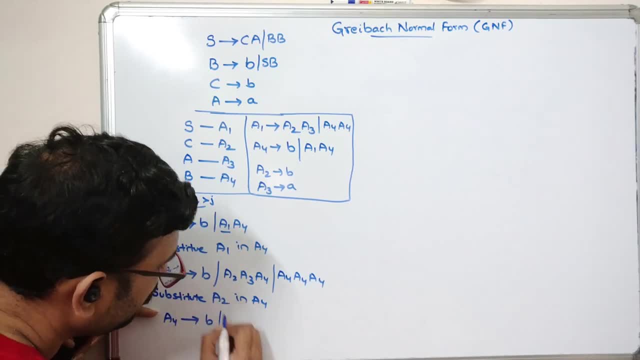 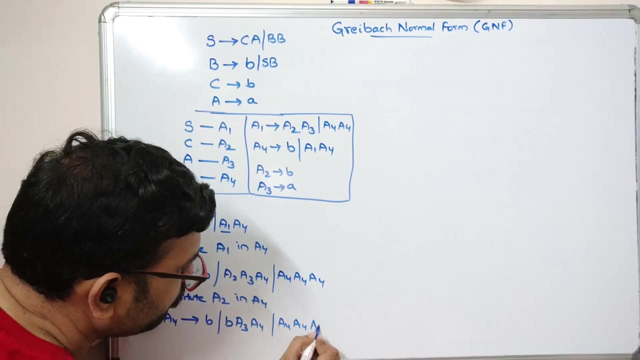 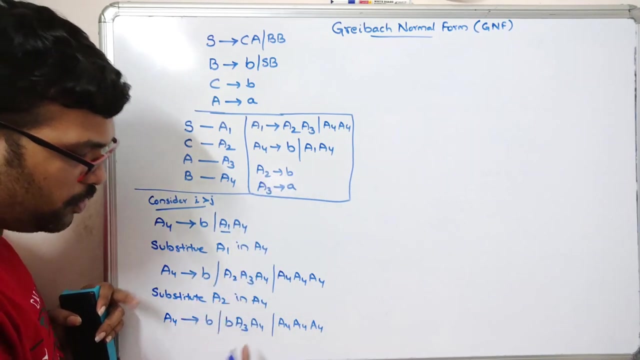 a4 tends to b or b, a3, a4, a4, a4, a4.. Hope you understood. We are just substituting a2 in a4. So a2 is replaced with b production, this one. So you can observe here: the first two productions are in g and f. 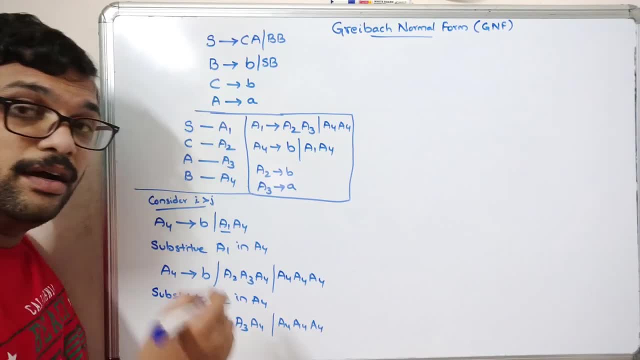 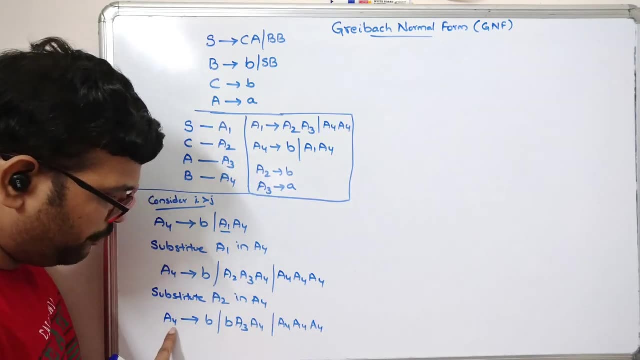 because first one is terminal and the second one is terminal, followed by two non-terminals. So that is also valid thing. And the third one a4,, a4, a4, you can observe a4 and a4. So 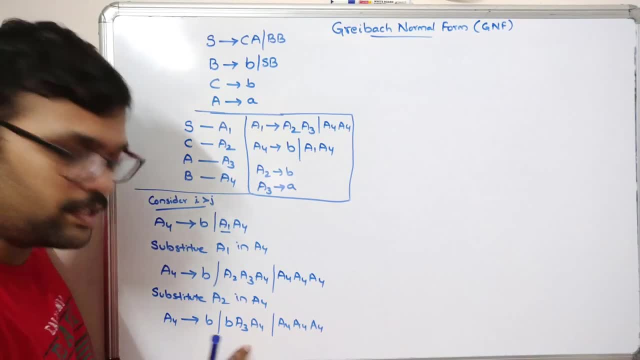 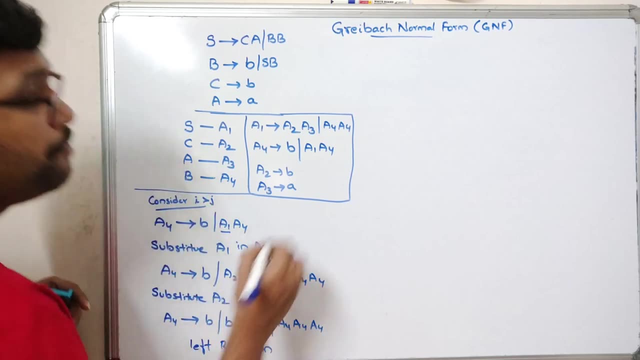 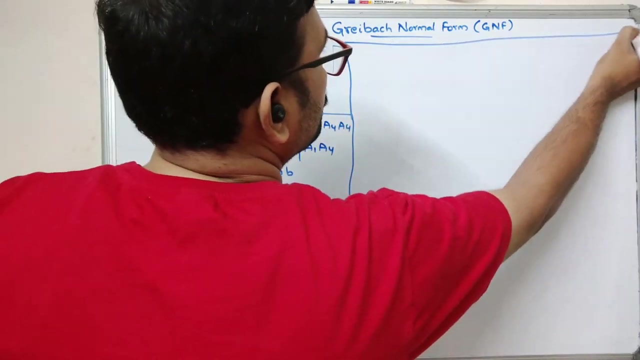 here there is a left recursion. Okay, here there is a left recursion. So here we are having left recursion, So we need to remove this left recursion. We need to remove this left recursion. So, after removing this left recursion you can see in the previous session. 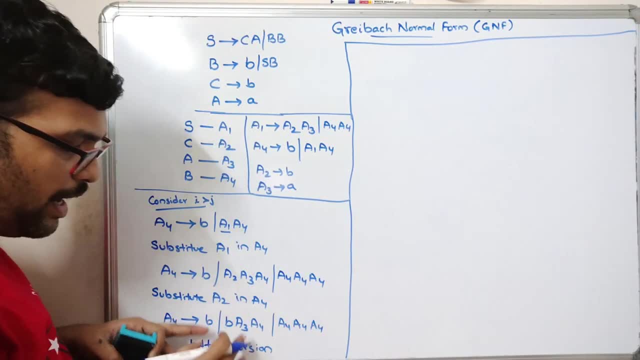 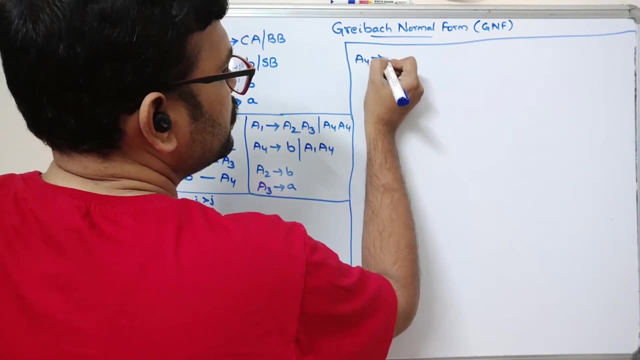 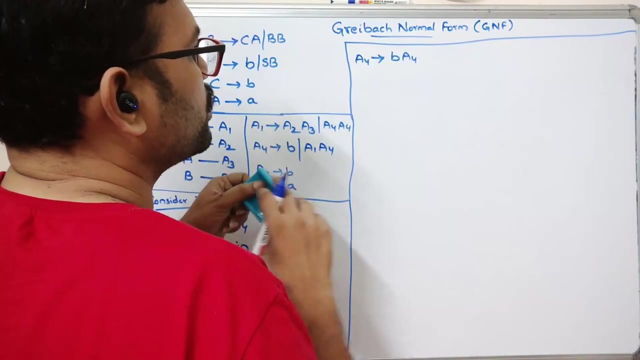 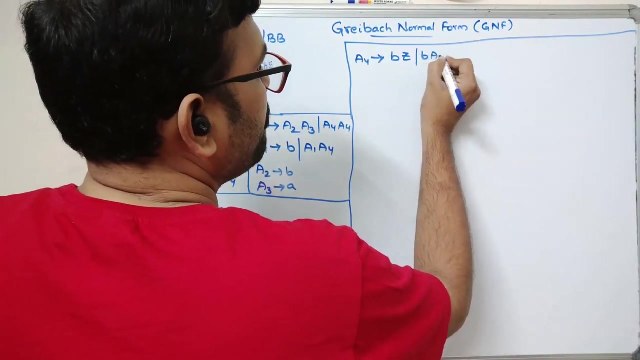 we have seen how to remove the left recursion. So first write down the productions which are not having the left recursion. So I will write here: a4 tends to b. I will go with the new production. I have to go with the new production, b, z or b, a3,, a4, z. 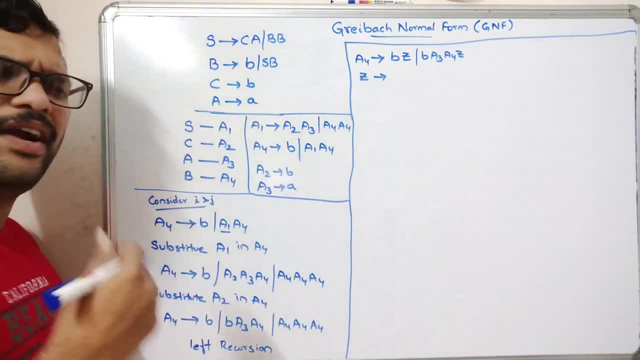 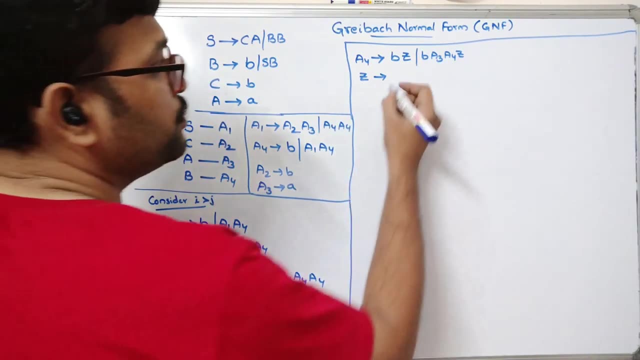 Okay, and we need to write the production for z. So instead of writing a4 dash, I am writing the z right. So z is equal to other than the left recursion. So you need to use this one a4,. 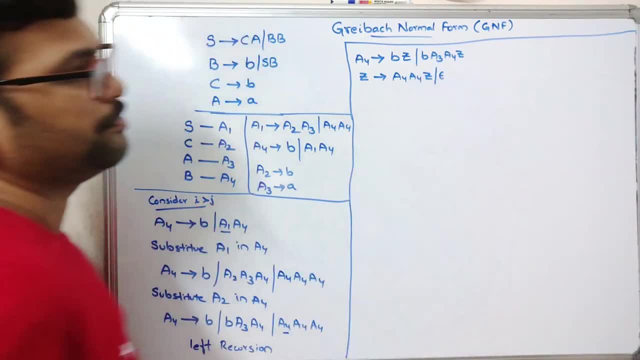 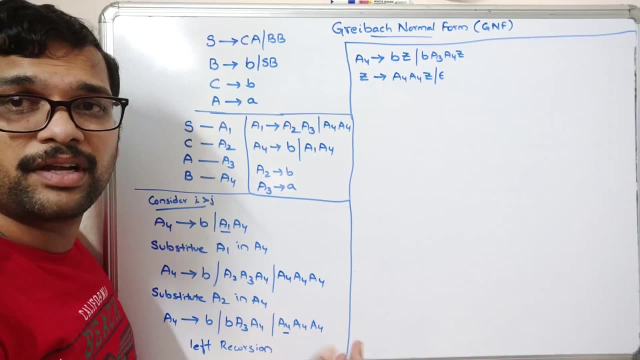 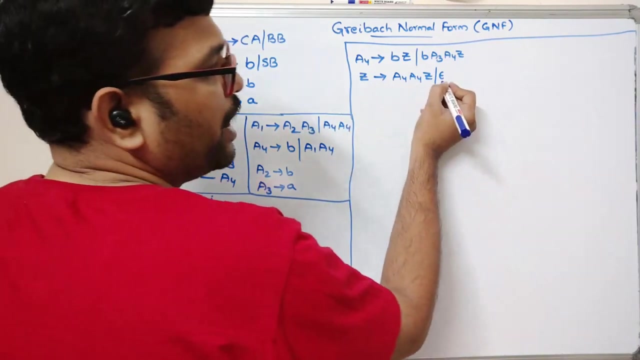 z or epsilon. Okay, a4, a4, z or epsilon. So this process we have already covered in the previous session. How can we remove the left recursion? So just, I will post the link in the description, You just follow that thing. So after removing this one, again we are having the 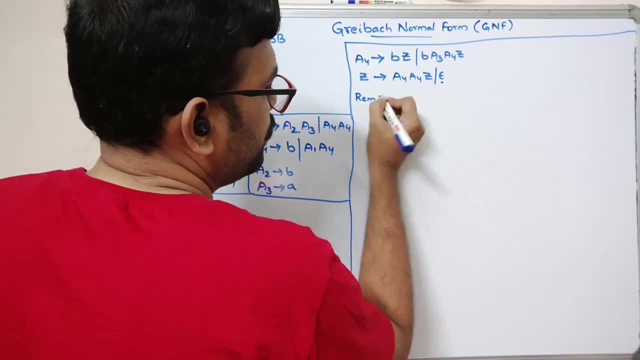 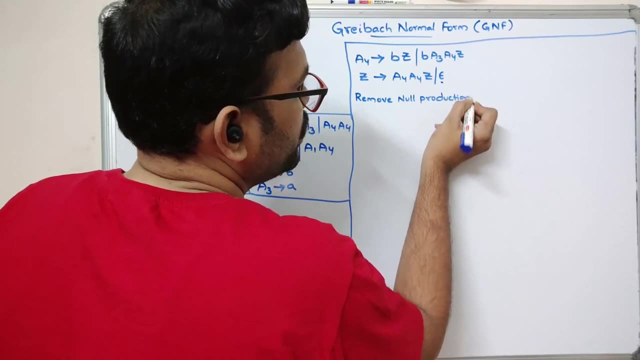 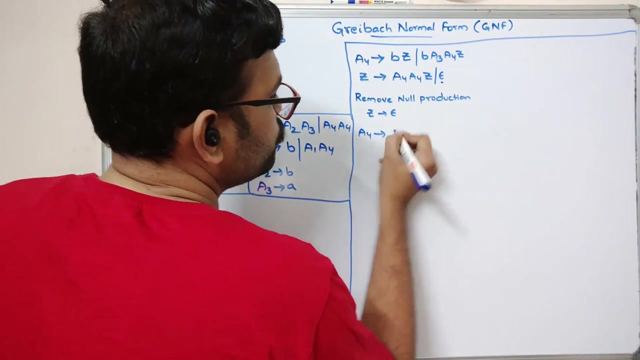 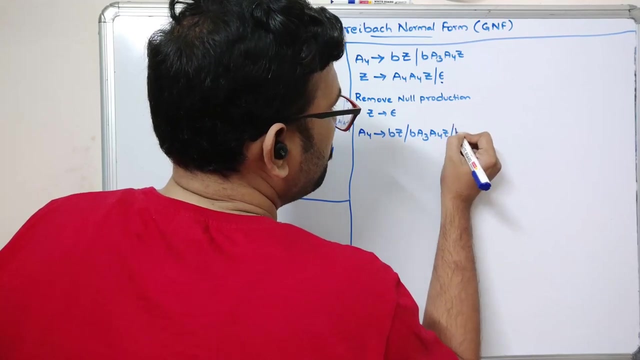 null production. So we need to remove null production, We need to remove the null production. So here null production is z tends to epsilon, Just apply here. So a4 tends to b, z, b, a3, a4, z, b, a3, a4. 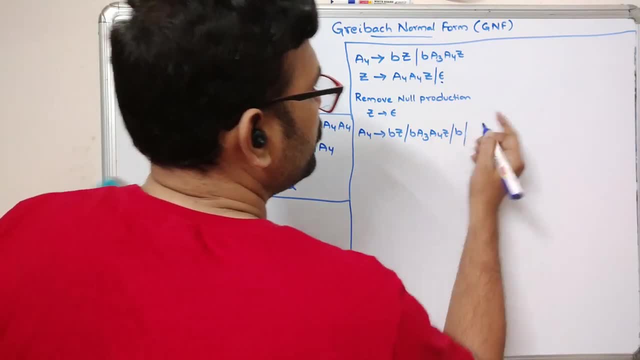 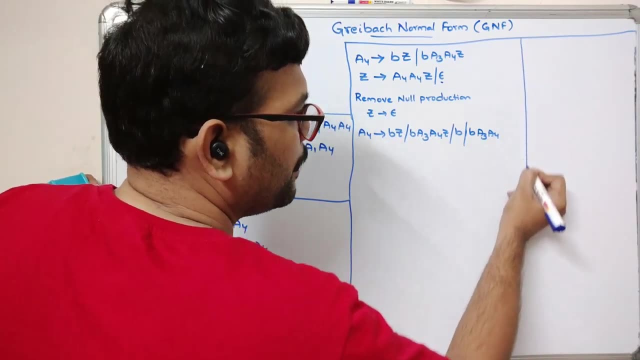 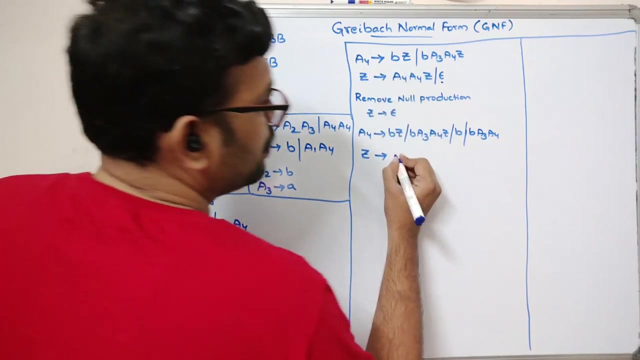 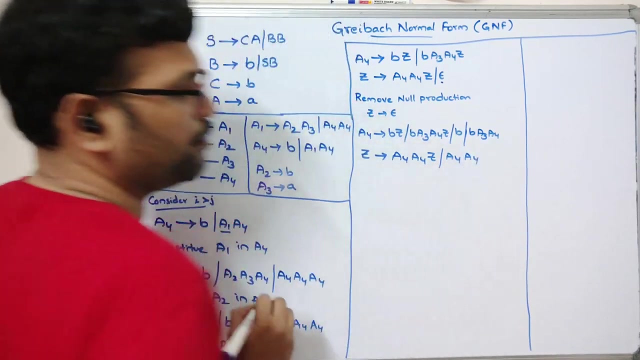 Sorry, here again we need to have the b, a3, a4.. Okay, b, a3, a4. Okay, Now again, z tends to write down the same thing: a4, a4, z or a4, a4, right, So hope you understood this one. 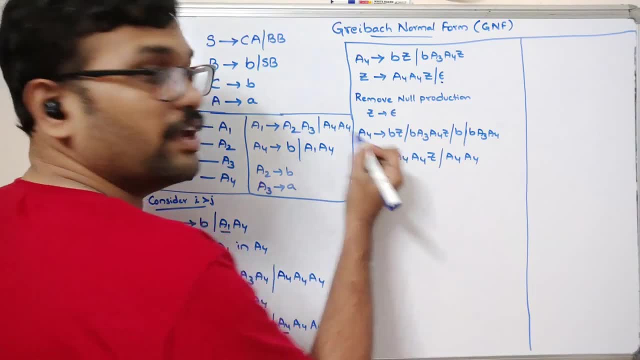 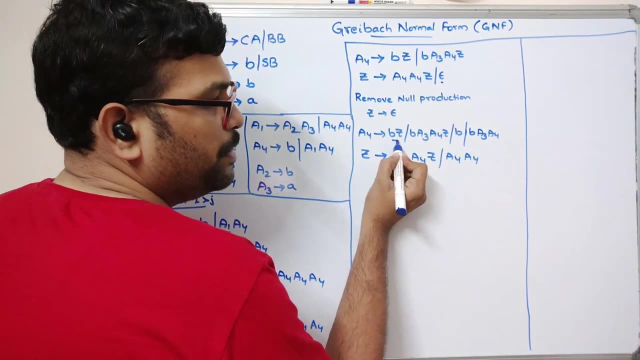 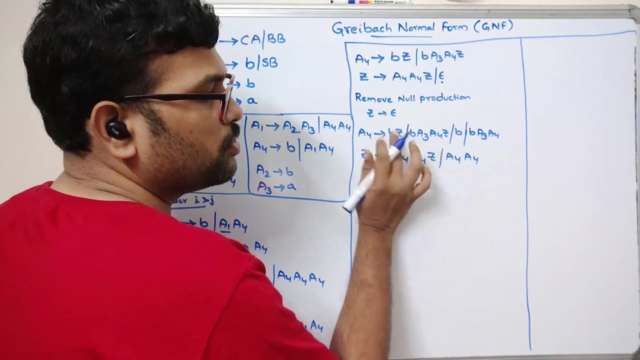 So now you can see the production of a4.. Here you can see the production of a4 is in GNF because here you can observe b, z, which is already in GNF Because it starts with a terminal, b, a3,, a4, z. It is also in GNF because it is also starting with terminal, followed by number of non-terminals and terminals. 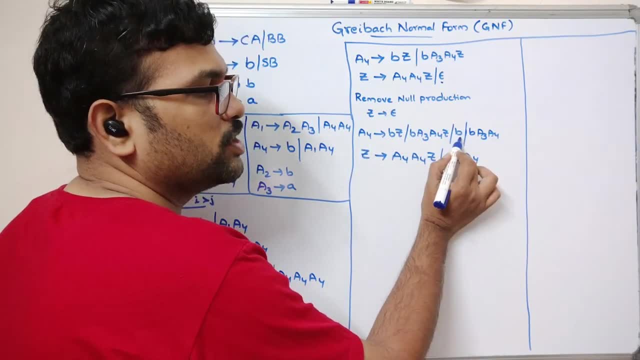 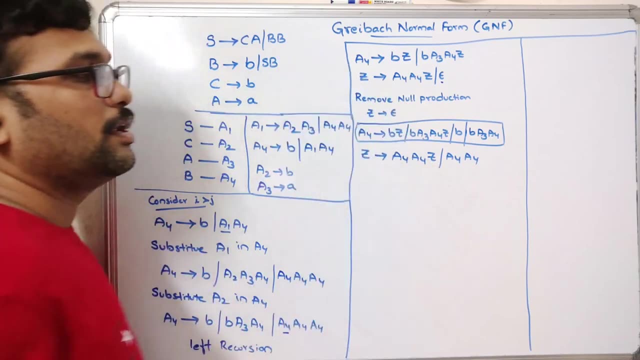 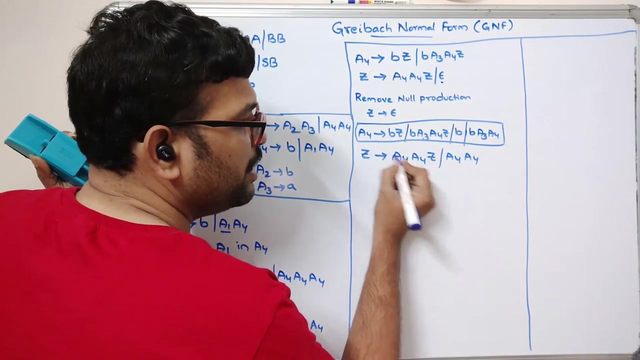 And again b, that means non-terminal, followed by a terminal. It is also in GNF, b a3, a4. So this one is in GNF Now. now, so consider, consider the general. So we need to replace a4 in GNF. 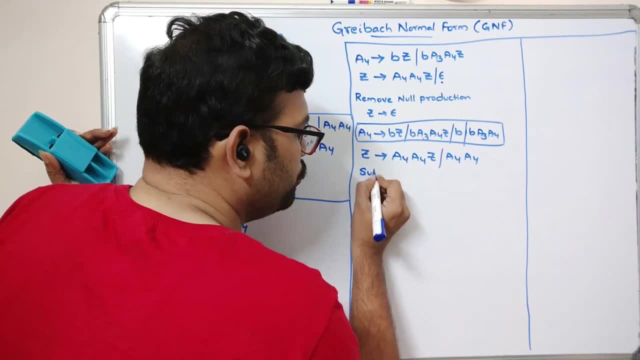 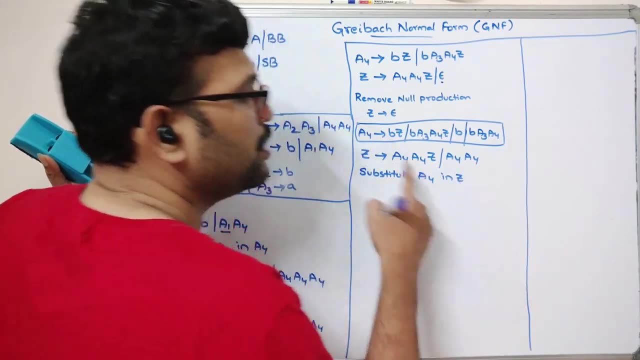 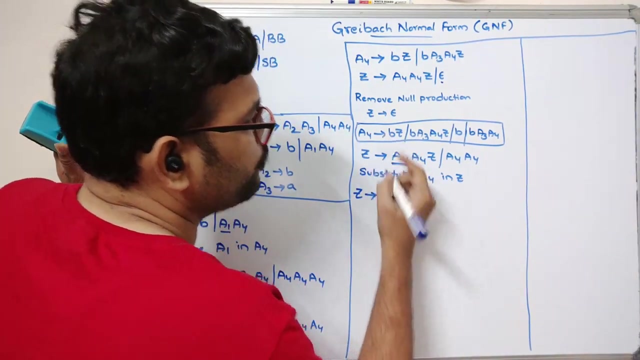 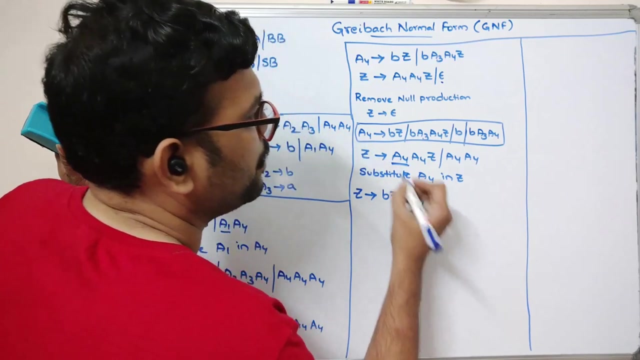 So substitute a4 in z so that z will be also in GNF. First let us consider the z. So I will replace this a4 with this one, So b z and write down a4, z, Next b, a3,, a4, z. 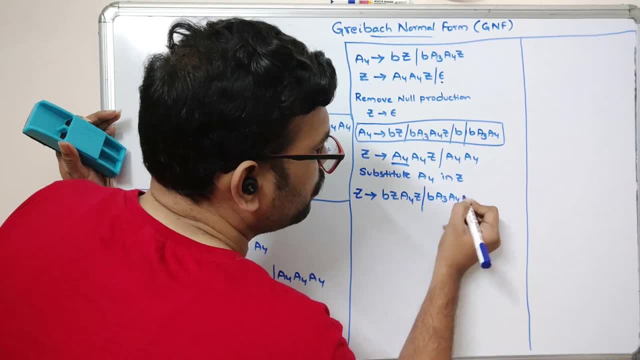 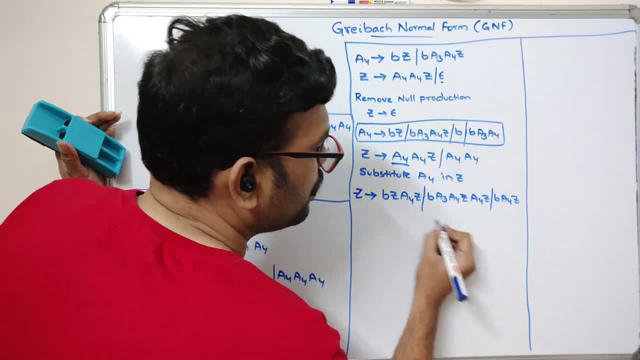 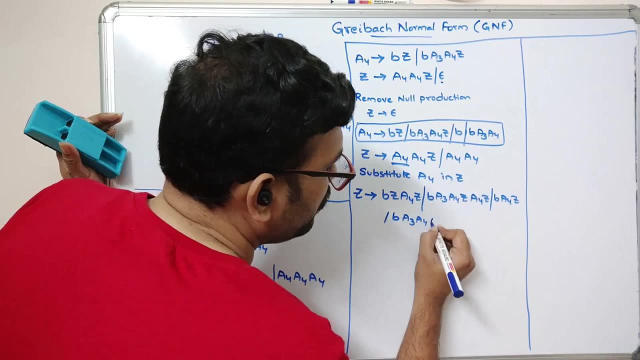 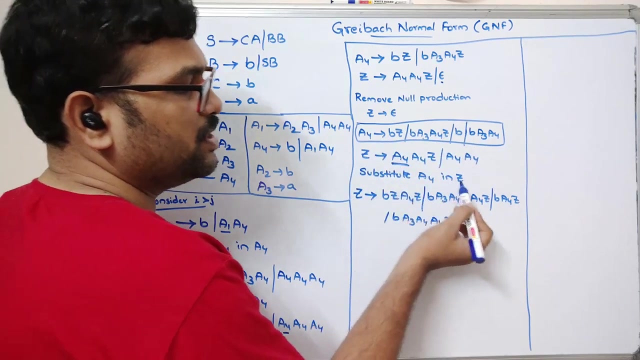 b a4, z. I will continue this one: b a3,, a4, and again a4, z. See once again. I am repeating: Just replace the a4 production here, Substitute a4 in z. 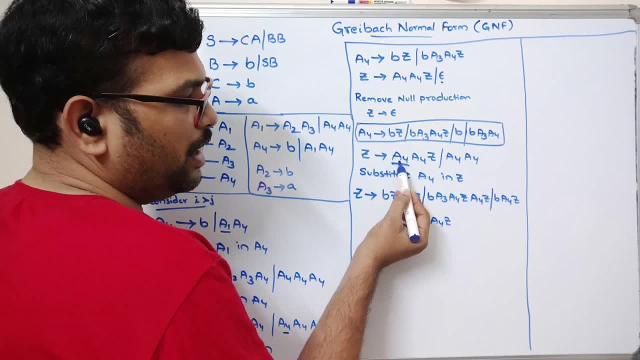 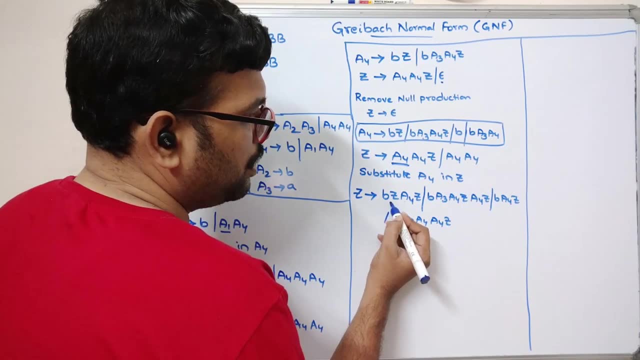 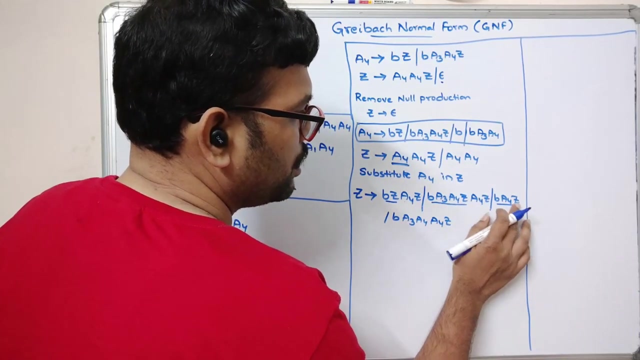 So first a4, right. So in the a4, I am writing b, z, followed by a4, z. So you can observe here: this is the A4 and this one is the A4 and this one, sorry here. 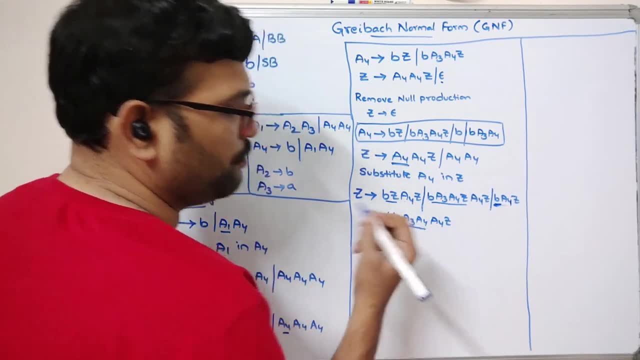 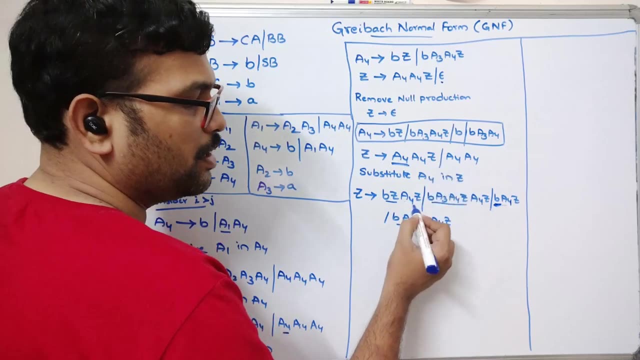 it is a terminal right. so this one is A4 and here this one is A4, right, I am replacing the A4 and I am keeping the rest of the string same. so A4, Z. now also, you have to replace. 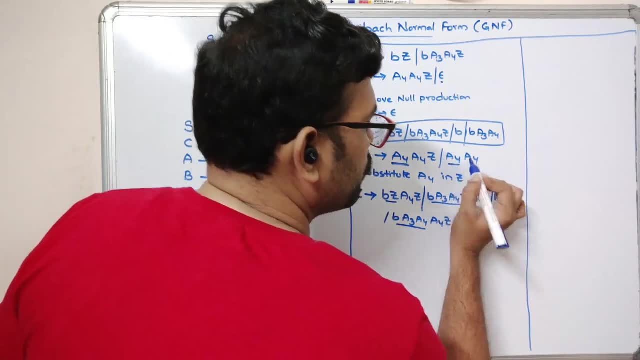 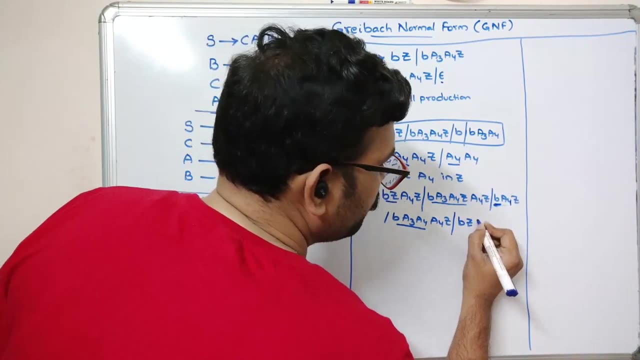 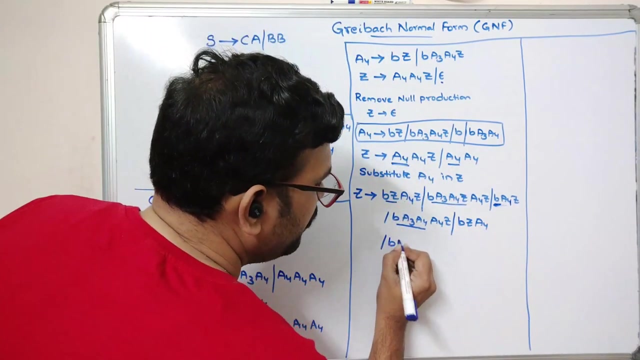 this one A4,, A4, so again you replace this A4, ok, I am continuing here. instead of A4, again go with the B, Z and use A4 here. ok, and see B, A3,, A4, Z and again write this. 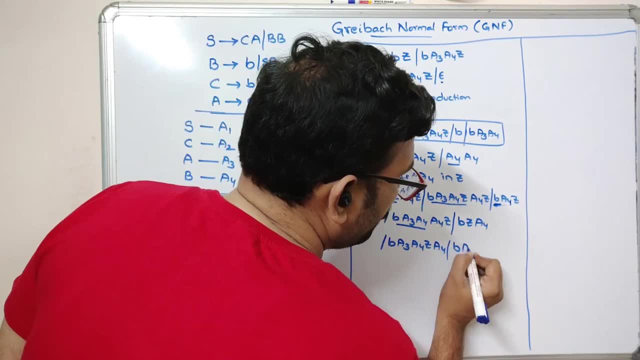 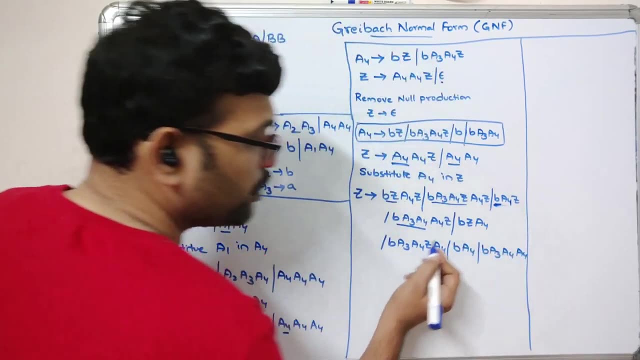 A4 here and B A4 here and B A3, A4.. A4, A4 here. So you can observe here: So this is A4 and this one is A4, this one is A4 and this. 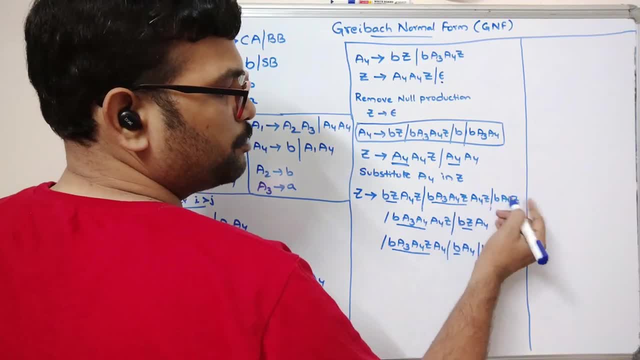 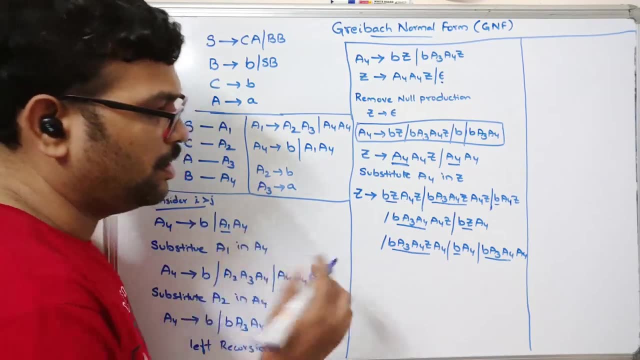 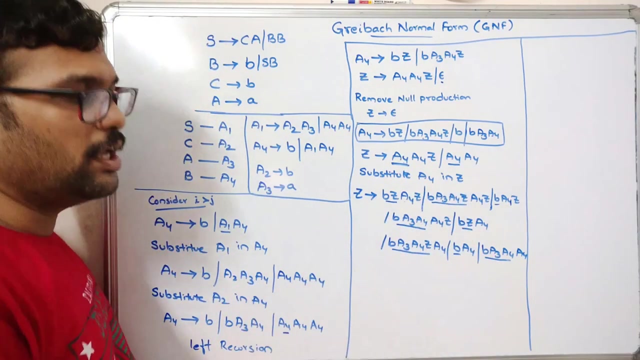 one is A4. So hope you understood this production. So the productions will be somewhat lengthy, but no problem, Just a substitution method. We are using the substitution method. So just substituting A4 in Z. We got this one and you can observe here. So Z is also in GNF, Z is also in GNF. 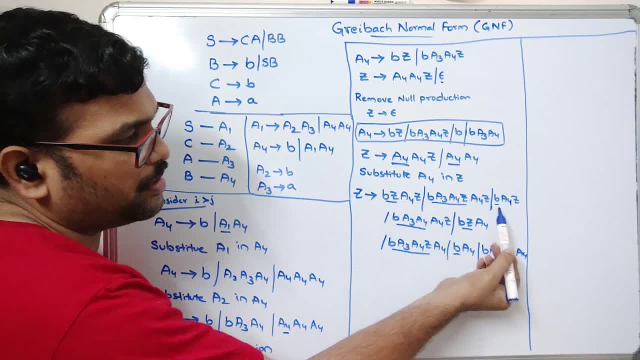 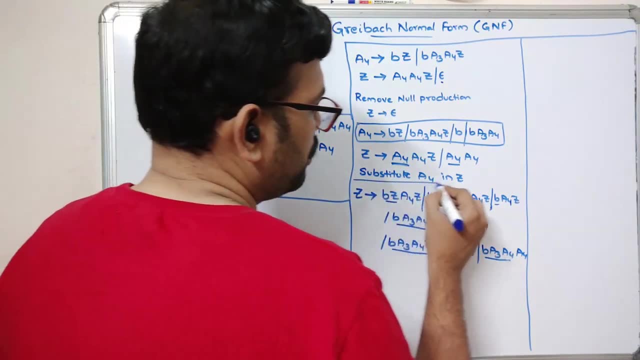 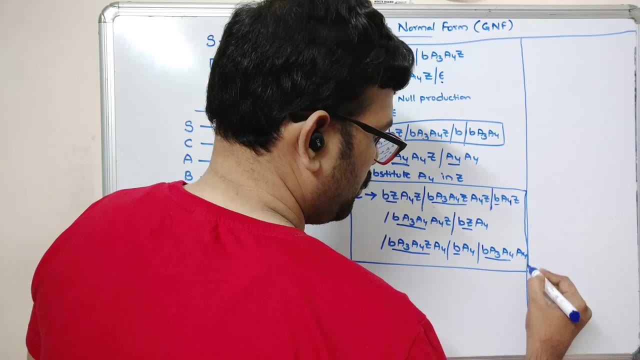 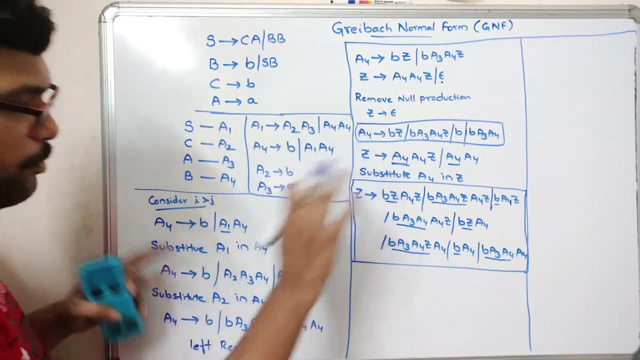 You can observe here It starts with the terminal terminal, terminal, terminal, terminal and here terminal, terminal and terminal. So Z is also in GNF Right Now. you can observe A4 and Z. Both are in GNF. A4 and Z, both are in GNF Right Now. consider: 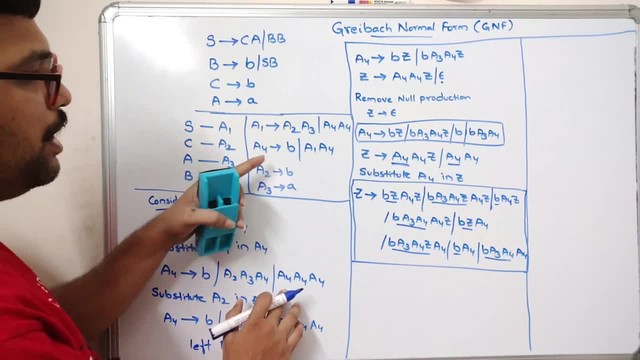 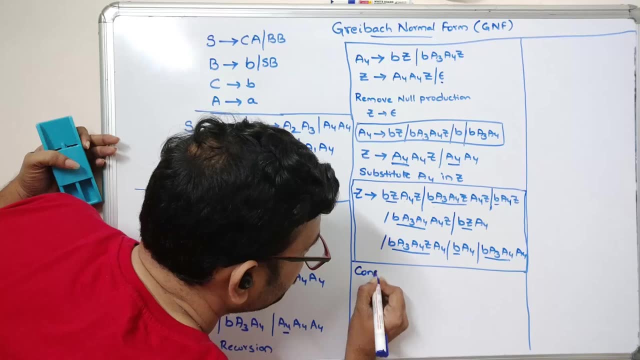 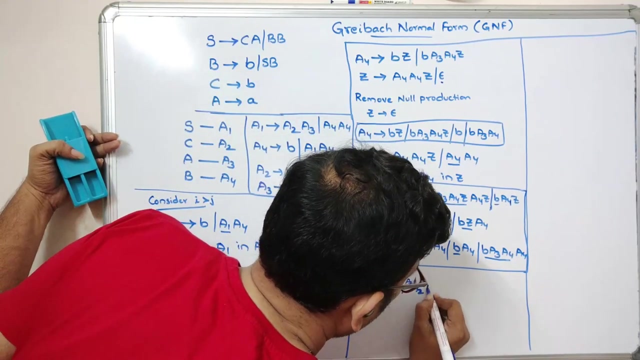 See, Now consider What is this one Right. A4 and Z are there. Now consider A1.. Okay, So consider the next one. That is, A1 tends to A2, A3, A4, A4. 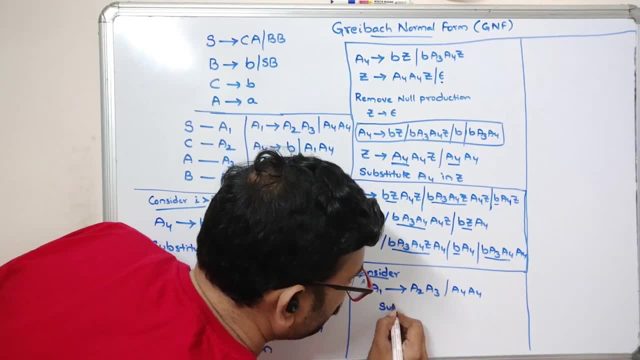 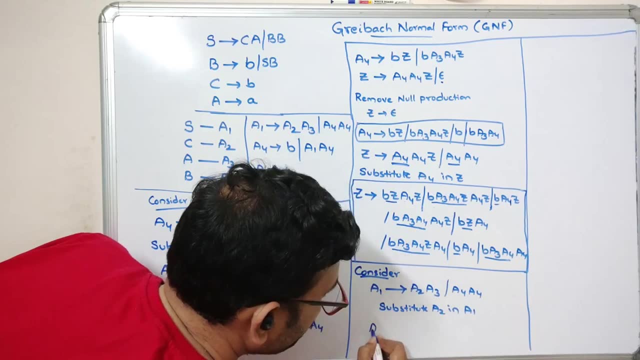 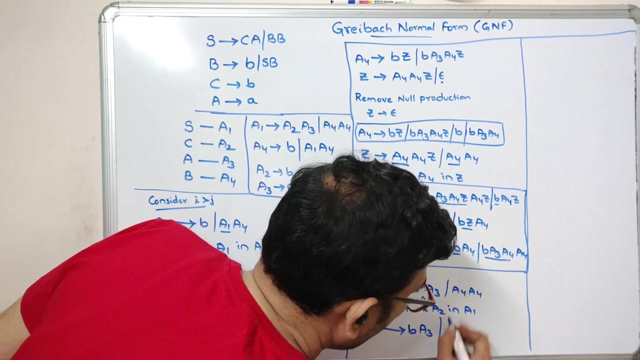 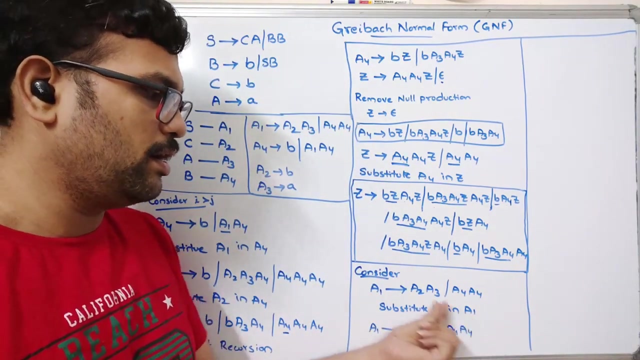 Okay, Substitute A2.. Substitute A2 in A1.. Okay, So we can have A1 tends to A2.. A2 is having B, So B, A3 and A4, A4.. Okay, Okay, We are just substituting A2 in A1.. Right, A2 in A1.. So in the A1 production we are having some. 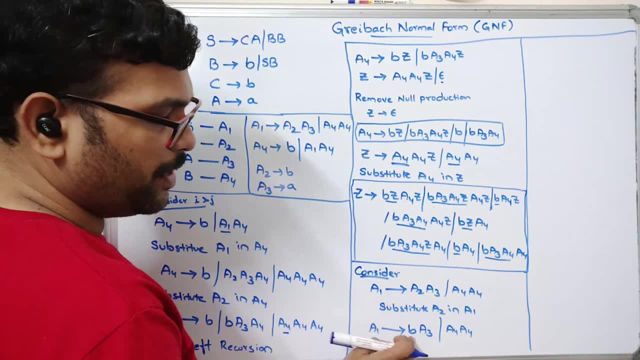 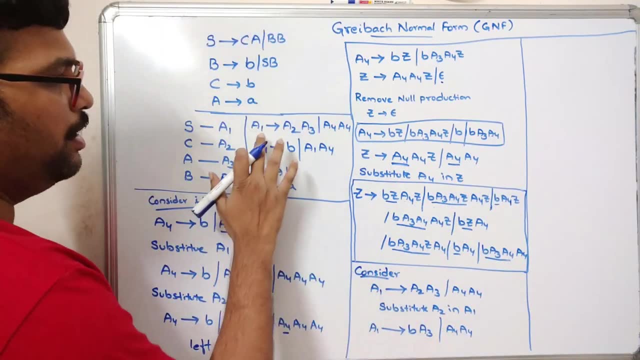 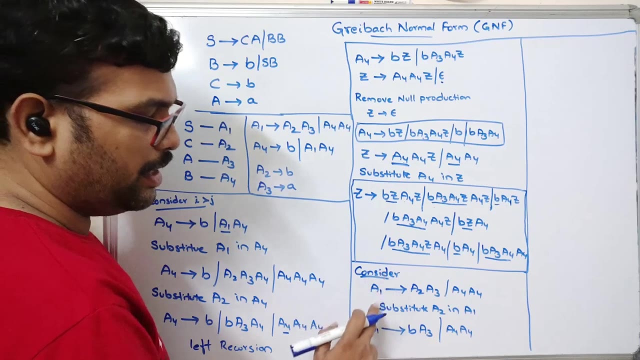 so A2 is having some B, so directly we are applying B A3, right now again we are. we can see here. so A4 is already in GNF Z is already in GNF A1, this production is in. 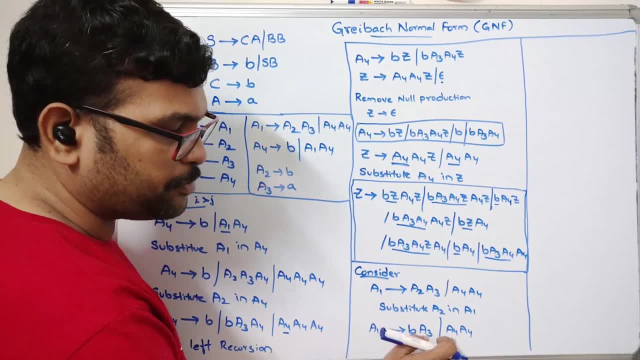 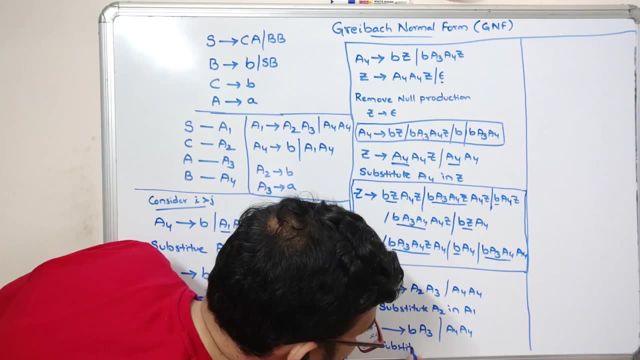 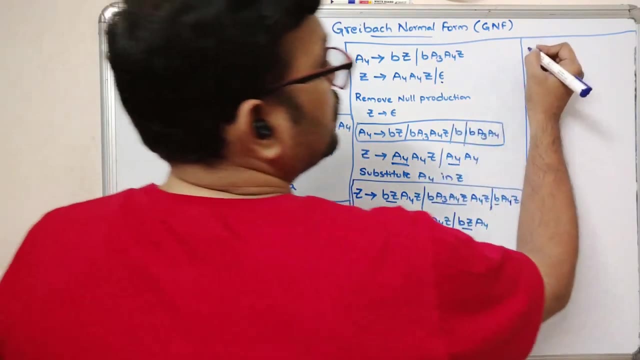 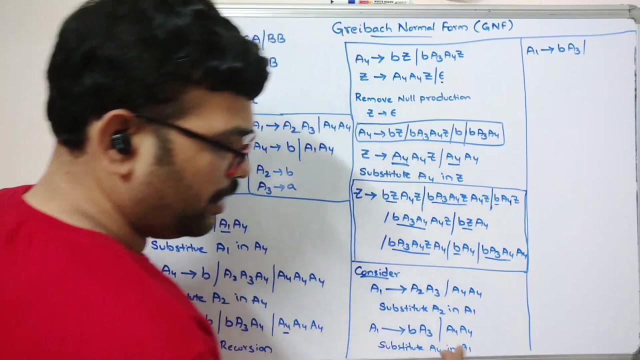 GNF and this production is not in GNF. so again, substitute A4 in A1,, substitute A4 in A1, right now see, A1 tends to. the first one is common B, A3, and instead of A4, we. 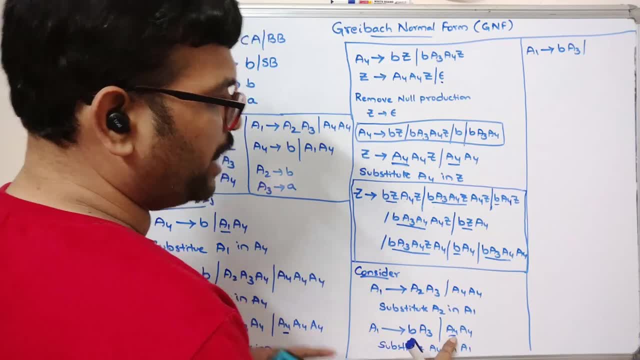 need to. we need to write the value of B and B1 in the raw zone. so we need to write the value of B and B1 in the raw zone. take half the value of B in the raw zone. take half production of A4. this one, this one should be substituted here, so BZ, BZ. 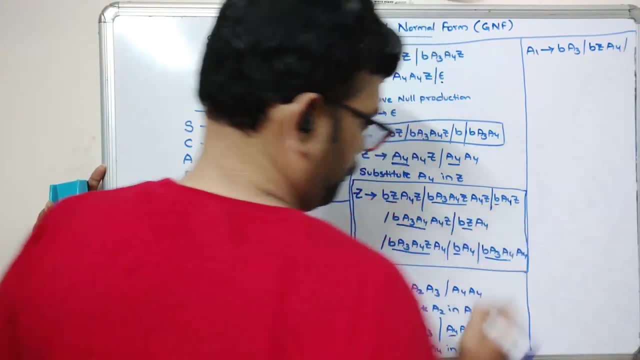 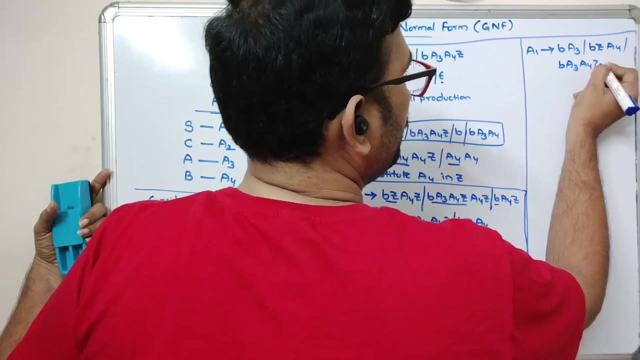 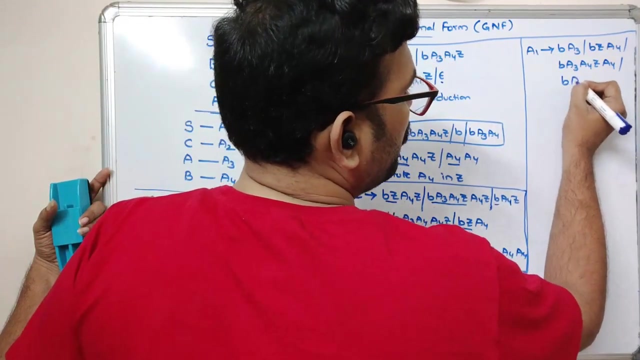 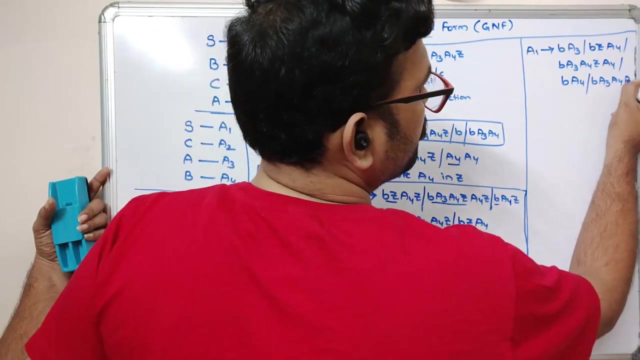 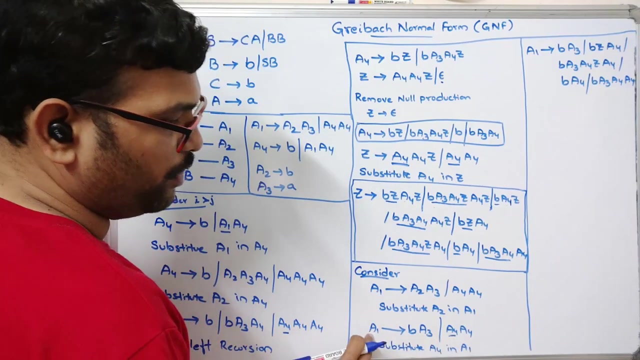 followed by A4. okay, then B, A3, A4, Z, followed by A4, next B, followed by A4, B followed by A3, A4 and Z4. right, see, just we are substituting A4 in A1, the production A4 in A1, so that you can observe: A1 is in G and F, so A1 tends to. 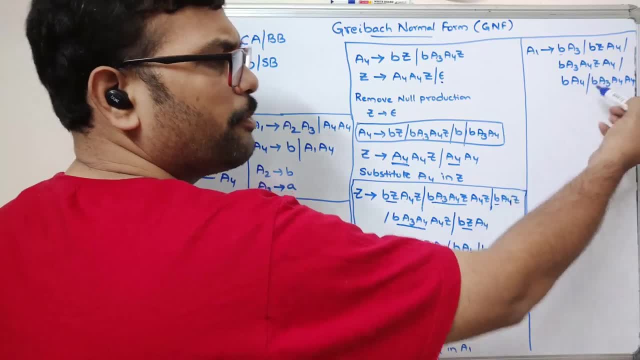 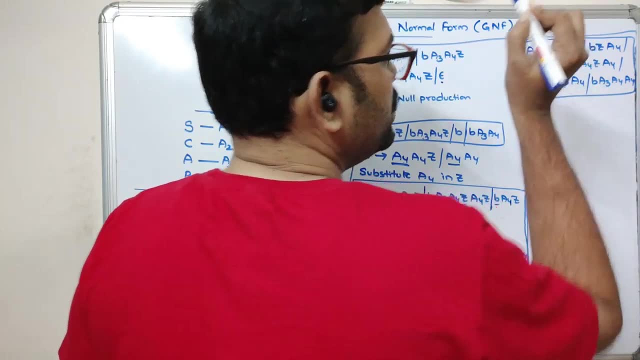 be A3, so B is terminal here. B is terminal, so every production starts with the terminal, so you can simply use this one. so A1 is also in G and F. okay, so A1 is also in G and F. so A1 is also in G and F. so A1 is also in G and F. 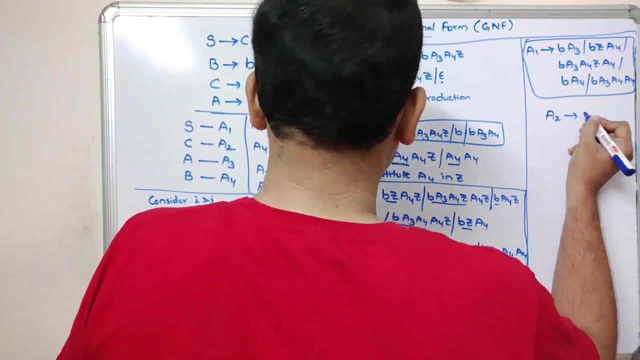 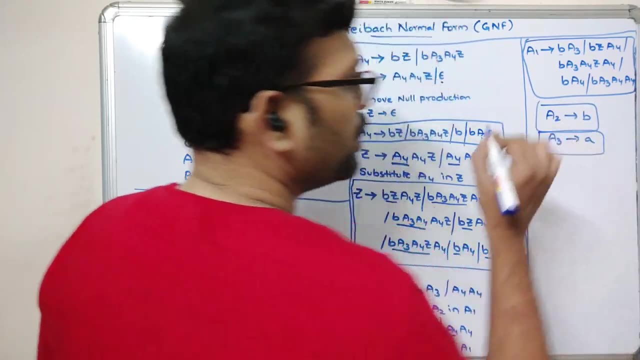 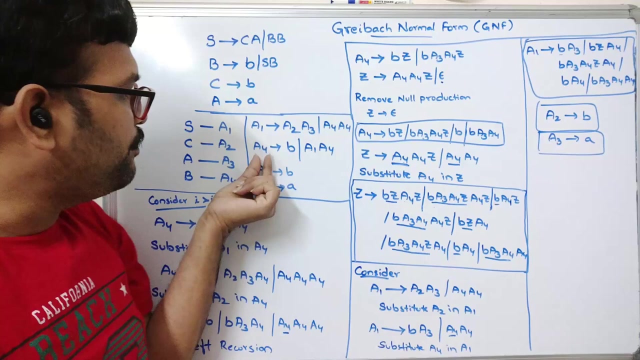 and automatically. we know that A2 tends to B and A3 tends to A, so both are in, also G and F. both are in G and F now you can observe here: so A1, A1 is already converted into a G and F, A4- A4 is again converted into a G and F, but A4 in the. 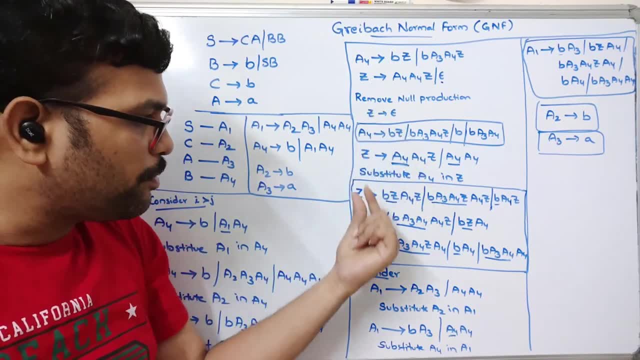 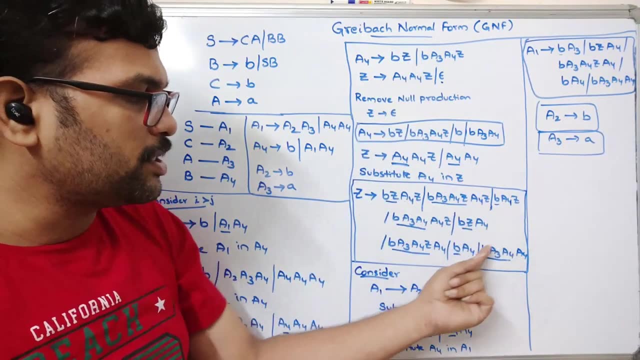 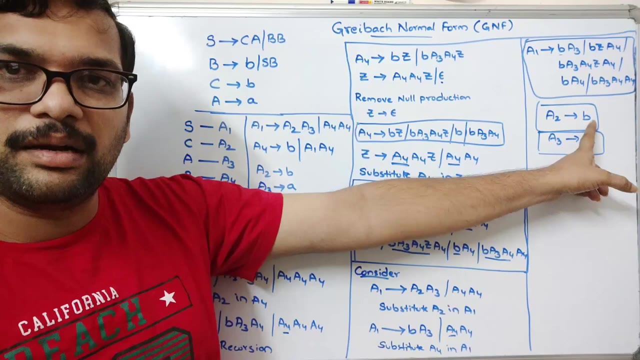 A4 production. we are having a non-terminal Z so we need to check the Z also. so Z also having the production, which is in G and F because all the productions starts with in terminal and coming to the A2, is already in G and F because it is generating the terminal and A3 is 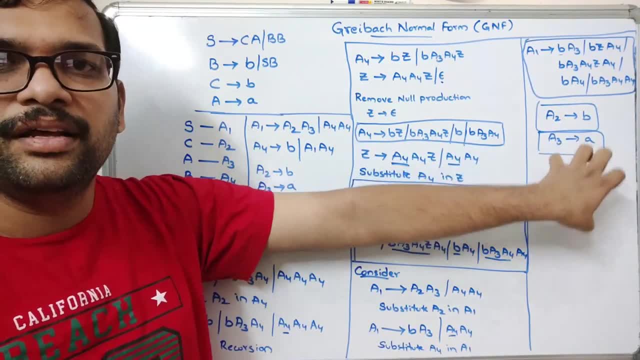 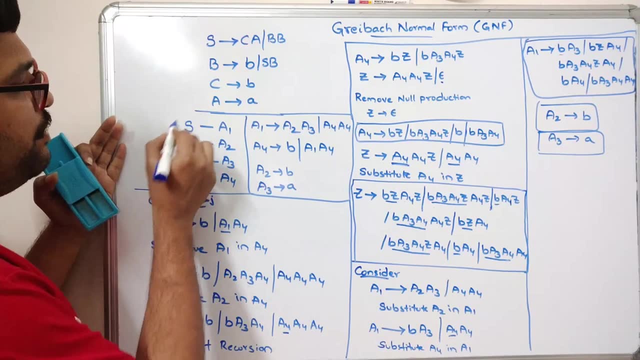 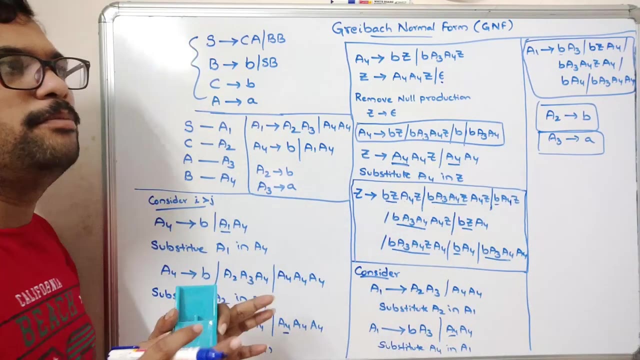 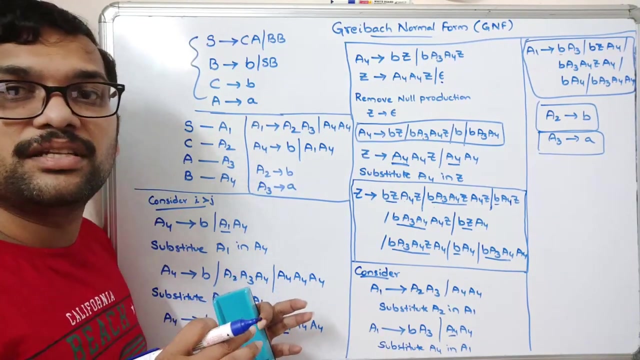 also generating a terminal so we can say that A3 is also in G and F. right? so after applying all the steps, we have converted the given CFG to G and F. so here one major problem is: the lengthy productions will be getting okay, don't worry about that, but here we are just using the substitution. 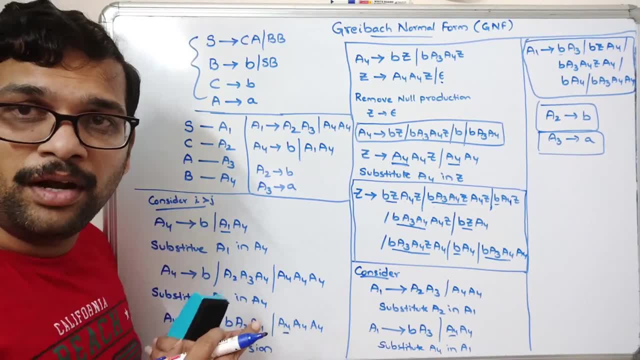 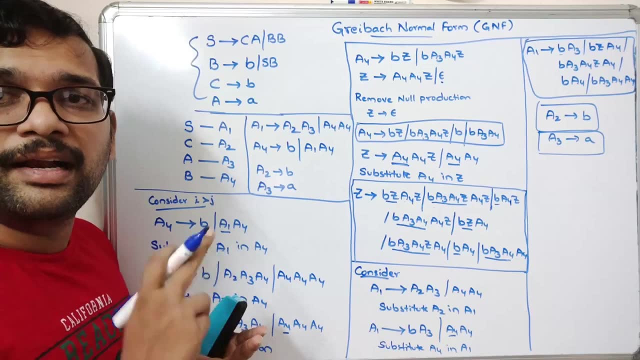 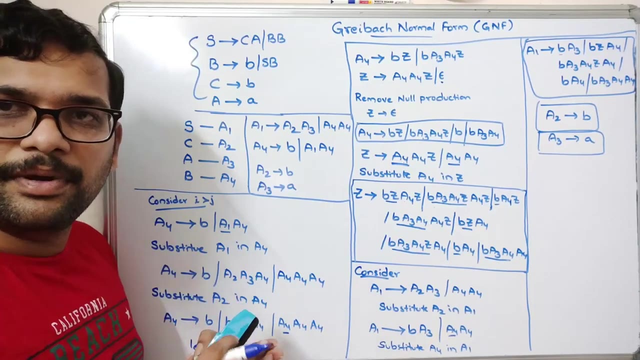 only you are using the substitution. so step one: the CFG should be in C and F, if not, you have to convert it. second step: rename all the non-terminals with the numerical variables, so the variable can be anything right. and the third step: consider AI tends to AJ, followed by anything. so consider I value and J value. 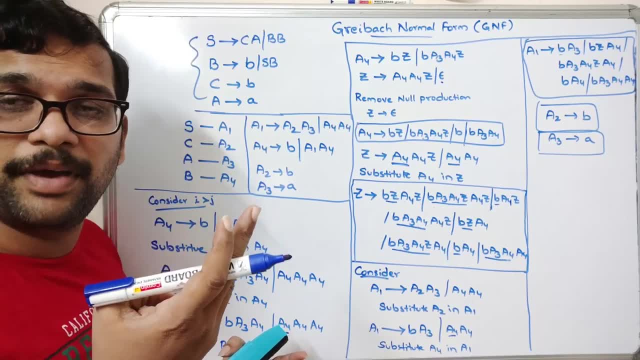 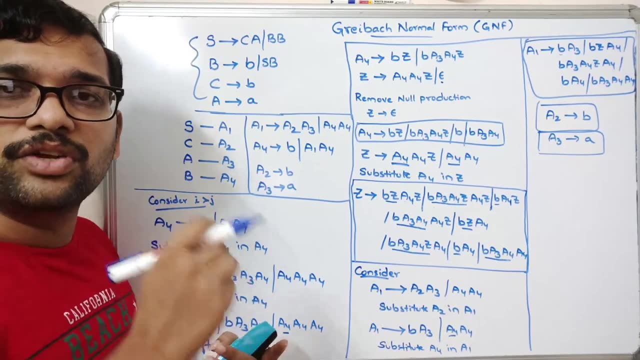 to compare the I value and J value. so there will be three possibilities in comparison: I less than J, I greater than J and I is equal to J. if I is equal to J, we can say it as a left recursion. so in the previous session we have seen the 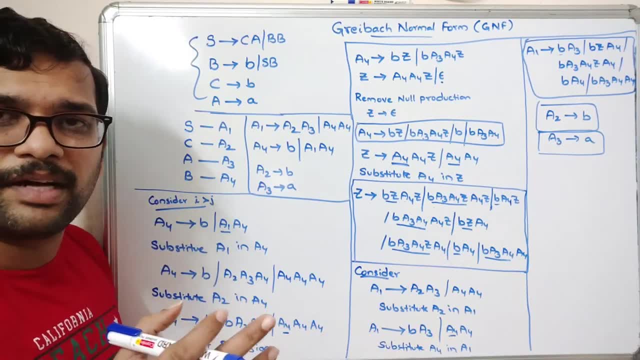 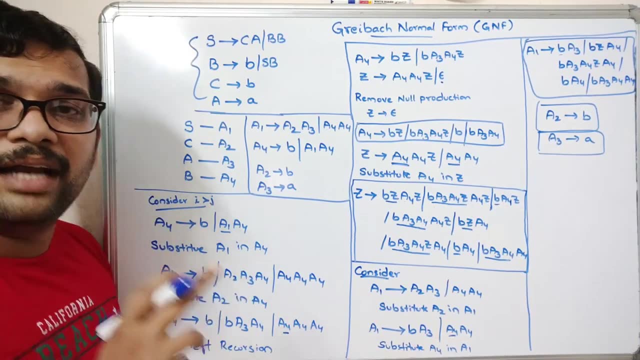 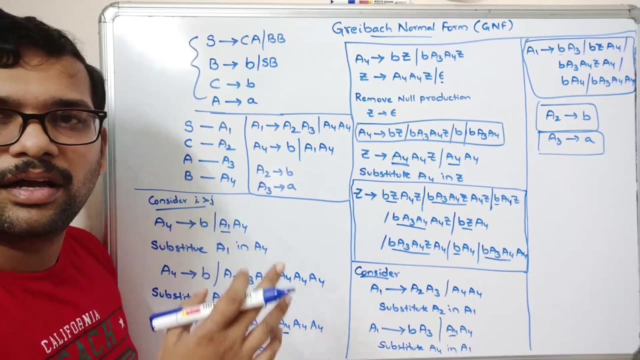 removal of left recursion, so which is not suitable for top down for our passing. so we have to remove the left recursion and consider the I greater than J and use the substitution and make sure the production is in G and F and from that again consider i less than j and again use the substitution and make the production that.